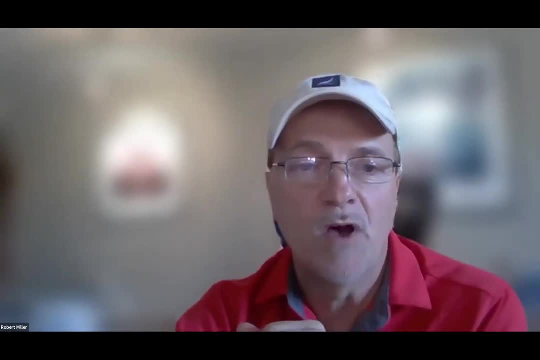 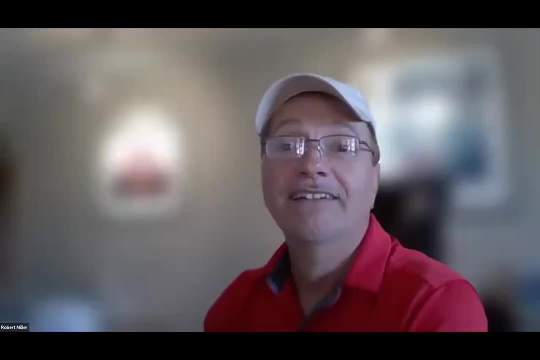 is talking to us today about. I don't see him on my list yet, but well, you know, Luke's here. Uh, pardon, Luke's Luke is here. Yeah, Luke's here. No, but John Jones, John, I'm here, John's. 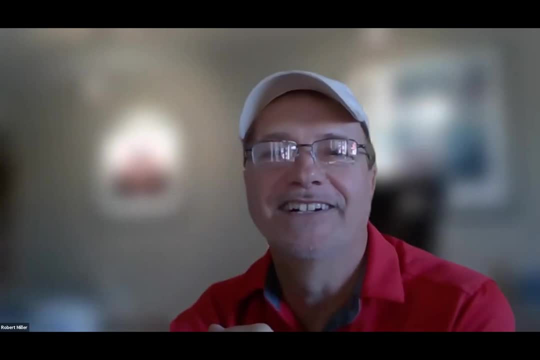 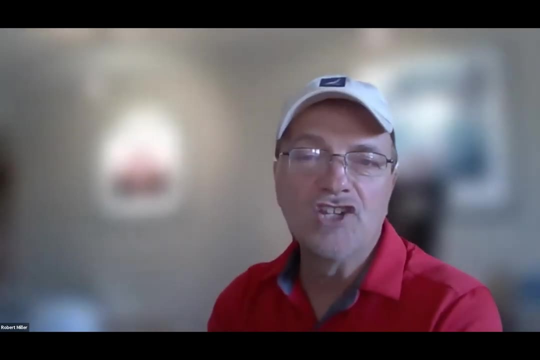 there. Very good. I'm sorry, My you, my screen, you guys go off my screen here. So thanks, John, for joining us today. So, uh, just just uh, John's new to our group. So, John, could you just give a very thin. 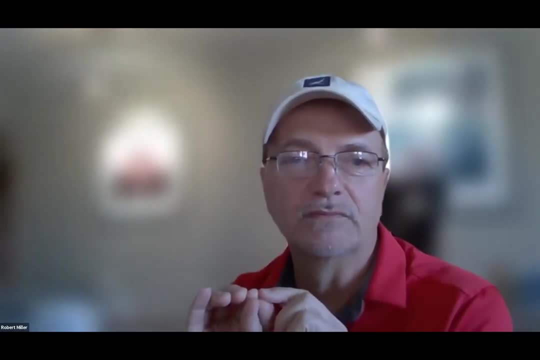 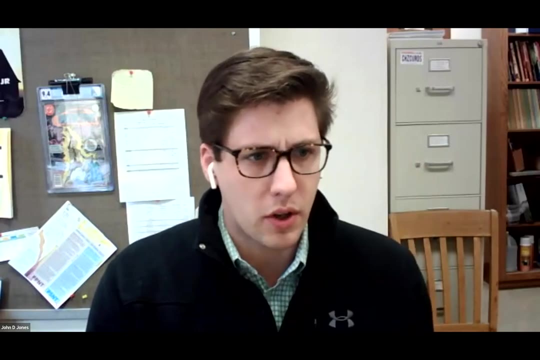 bio about yourself. Sure, Thanks, Bob. Um, so the the work Bob was talking about was part of my master's and PhD work at Iowa state. Um, so we were looking at a few different things about the recommendations that. um, I kind of caught when I came on Luke was talking about. 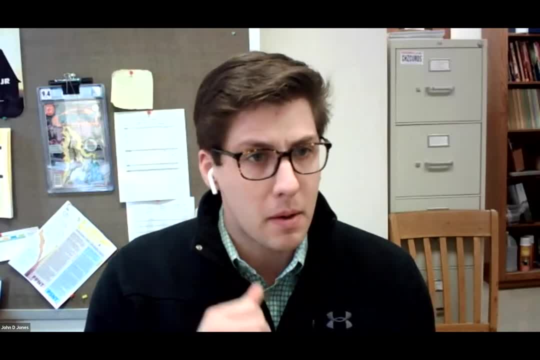 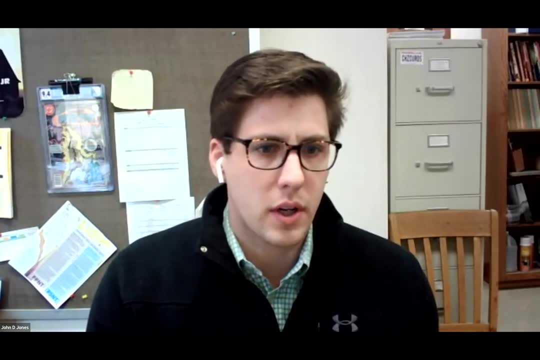 um there, we didn't know why and we wanted to investigate. um. I'm in Madison, Wisconsin at UW in the soil science department um staff uh academic researcher, So I cover uh in soil, fertility, nutrient management, So anything related to PK, Lyme micros and uh a little. 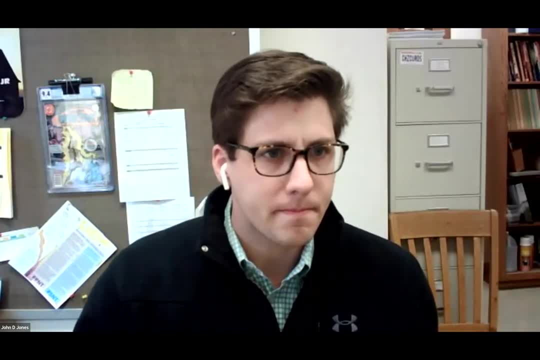 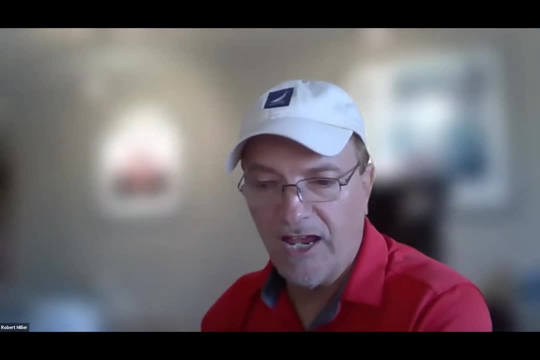 bit of nitrogen, uh projects on alternative forage crops. Very good, Thank you very much for that, John. So, so, uh, the way we're going to work the rest of the agenda today, we're going to jump on his presentation on soil acidity. 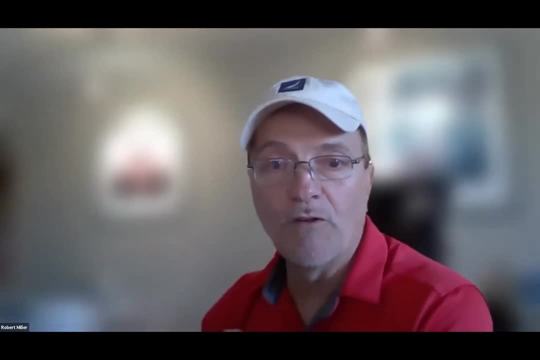 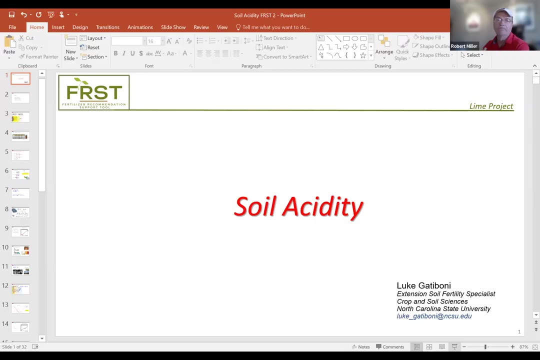 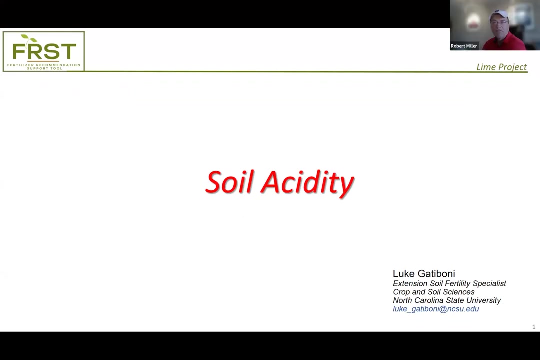 Then I have a few comments at the end and we'll go from there. So I'm going to hand the ball over to Luke. You got your sharing up right, Luke? Yeah, Okay, Are you seeing it right in presentation mode? Yes, everybody see it. 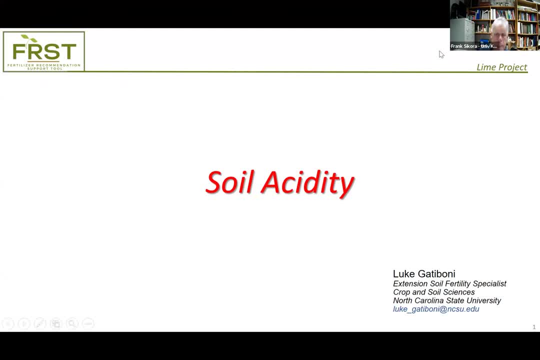 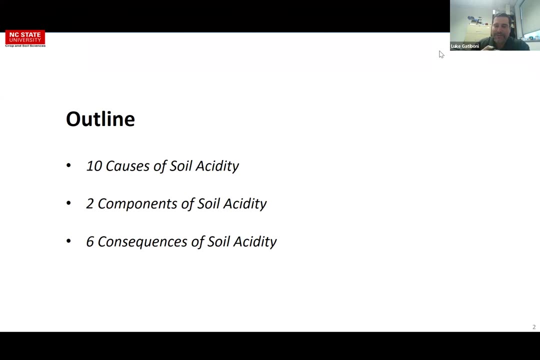 Yes, yes, Hey, Okay, And so this presentation. Bob asked me to do a basic presentation about soil acidity And during this presentation we will talk about the causes of soil acidity and I will talk about the 10 causes, the most common causes of soil acidity. 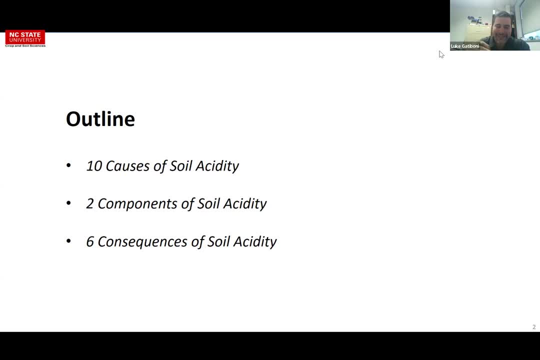 the two components and the six consequences that I can list of the bad consequences of soil acidity, And so I don't think we'll have too much time in this. It's a long class when I have soil fertility with my students and I've been started. 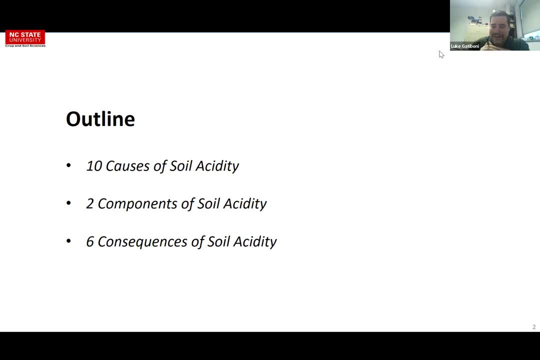 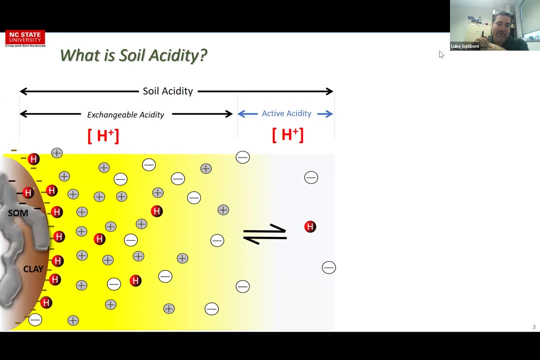 I'm trying to condense this in a quick presentation And so I move fast and we can discuss in the end if you have any questions. And the first thing: when you are talking about soil acidity, you are talking about hydrogen, We are talking the acidity is always high. 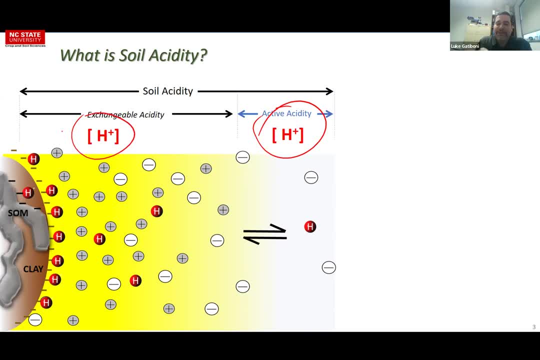 So we are talking about hydrogen. We are talking: the acidity is always high. So we are talking, the acidity is always high And we have two compartments in the soil that we can have the hydrogens. We have the active acidity that you can measure in the soil. 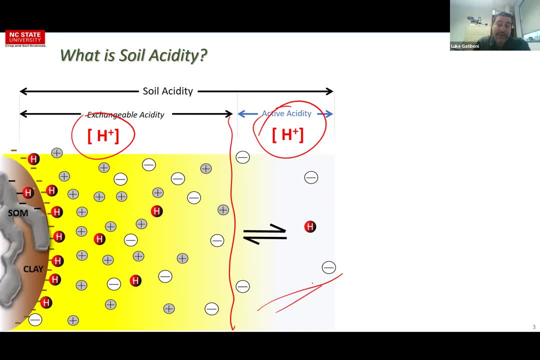 with the pH and it's located in the soil solution And we have those hydrogens that we have in the CEC in the solid phase of the soil And these hydrogens are buffering the book solution And but sometimes when we have, the pH is very low. 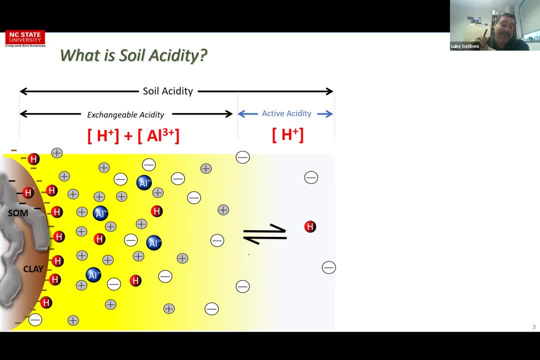 we have another component of these acidity that we can consider, the aluminum, as also a component of soil acidity, because this aluminum will go to the book solution, will react with water and will generate more hydrogens, And so if you have a really acid soil, 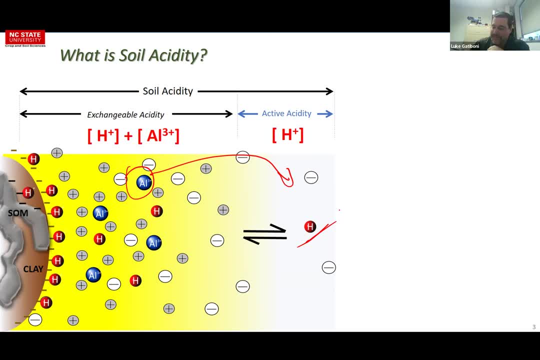 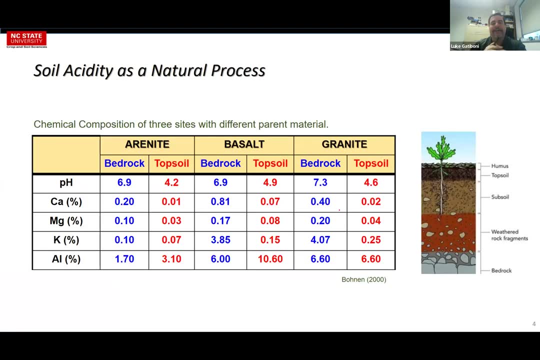 aluminum could be considered as a component of the acidity, And we will talk about aluminum in this presentation, later in this presentation. And the first thing, the soil acidity or the soil acidification is a natural process. It's a natural process. 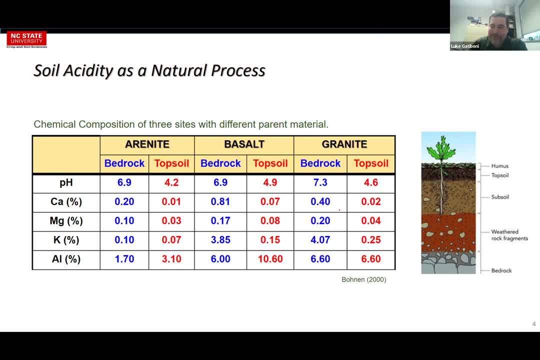 And you can see this guy. I like to present this slide because this guy got a ground rock from the bedrock and got the top soil in different sites, different types of parent materials, And he measured the pH: calcium, magnesium, potassium. 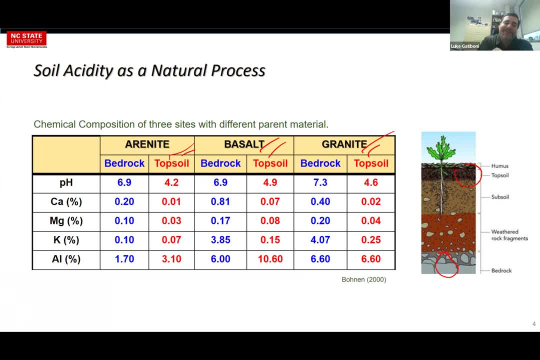 and aluminum in the rock and in the top soil And you can see that during the weathering process in the soil formation, the pH will drop in all these soils. the calcium, magnesium and potassium will drop in all these soils, because we lose these elements with time. 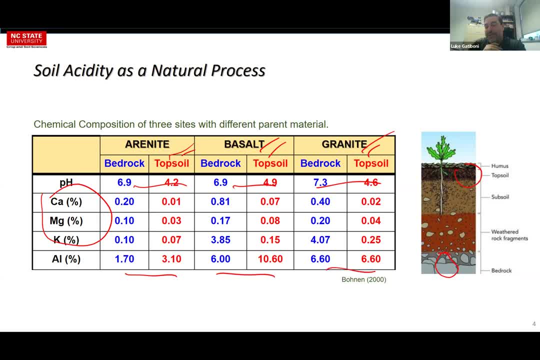 and the aluminum percentage will increase. It means that this is a natural process that is occurring in the soil, that we are increasing aluminum and hydrogen and you are decreasing these other cations during the soil formation, And all of these is related to acidity. 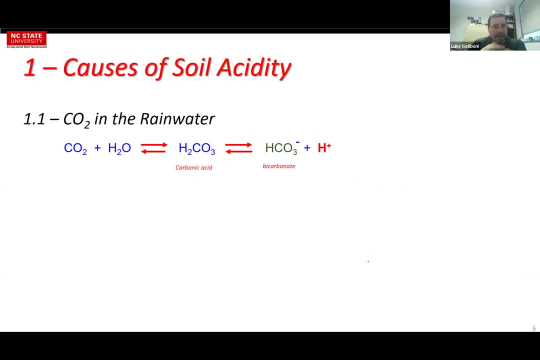 Talking about the causes of acidity, and I told you that I will mention about 10 different causes of acidity. We'll start with the CO2 in the rainwater. We have the CO2 in the atmosphere and this CO2 will react with the rainwater. 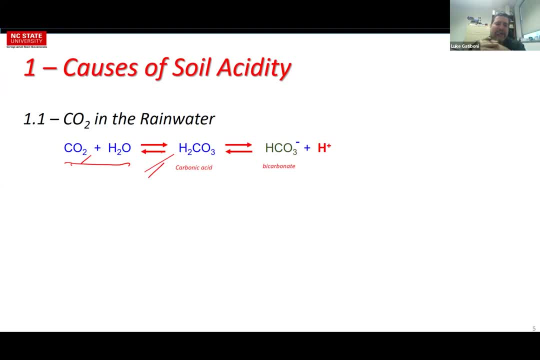 And we have this equilibrium, chemical equilibrium, and we can form a little bit of carbonic acid in the rainwater, And this carbonic acid also has another equilibrium that will split in a little bit of bicarbonate and hydrogen. And so when we think about the rainwater, 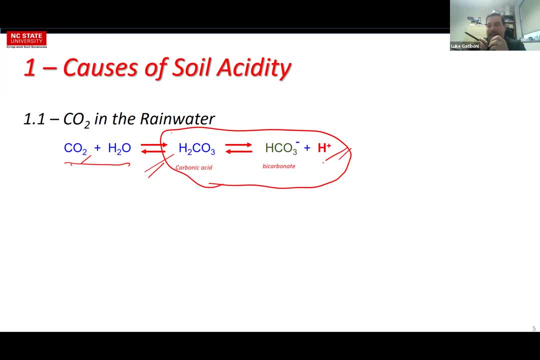 it's common to have, the pH of the rainwater is a little bit acidic because we have a little bit of hydrogen in the water coming from this process, this equilibrium, chemical equilibrium process, The same as will occur in the soil atmosphere: We have air inside the soil and we have CO2.. 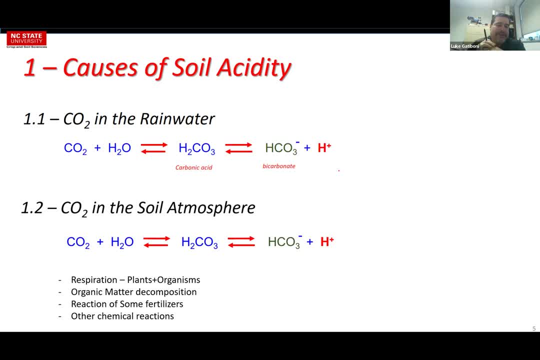 This CO2 comes from the respiration of plant and organisms. It comes from the organic matter decomposition reaction of some fertilizer. all of these and other things can produce some CO2 in the soil atmosphere And we have exactly the same reaction in the soil atmosphere. 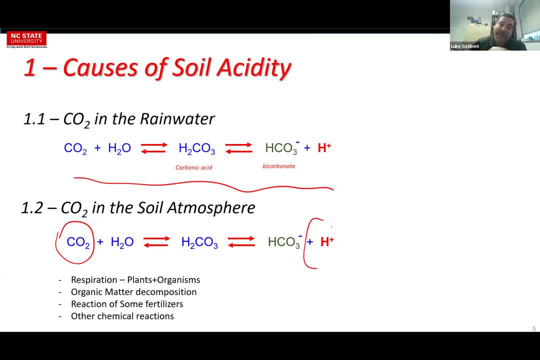 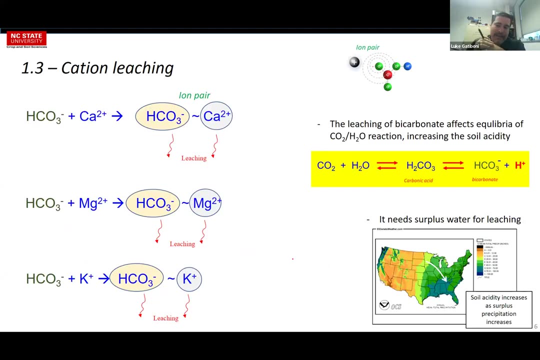 that we have in the rainwater, And so again, we can produce some hydrogen in this process, But the amount of hydrogen is very small in this equilibrium because the carbonic acid is a weak acid. The next thing is cation: leaching And cation. 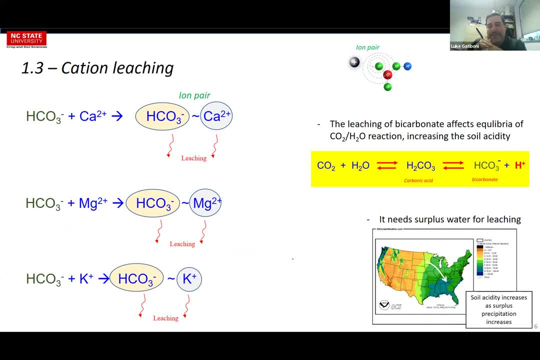 leaching is tricky because cation leaching is a consequence of the soil acidification, but it is also a cause of soil acidification. What drives the cation leaching? The? The cation leaching is when we have calcium magnesium. 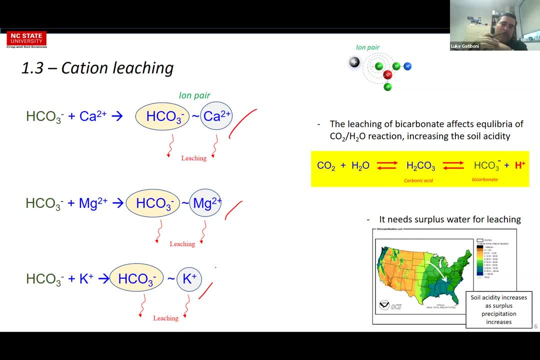 and potassium, and also sodium, of course, but I will focus in our elements that are important for plants. We have calcium, magnesium, potassium that can be leached from the soil solution if you have a lot of water, if you have more precipitation than evapotranspiration. 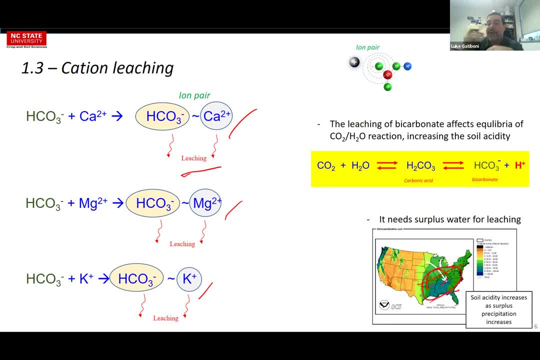 So you can see, in these regions of the United States where we have these, the rainfall is higher than the evapotranspiration. you can have movement of water downwards in the soil profile, and so we can move calcium, magnesium and potassium. 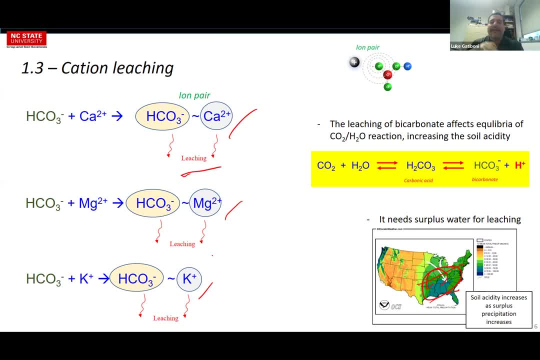 And the interesting thing is that this calcium, magnesium and potassium, they are not moving alone, They can move in ion pairs with bicarbonate, And the ion pairs is just because we have this guy that is a cation, we have this anion. 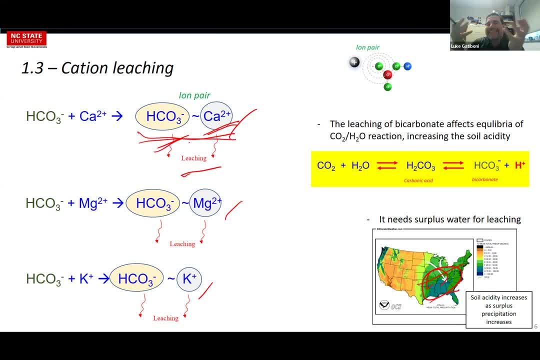 in the solution and they will be attracted by each other. It's not a chemical bond, but they are just attracted. It will decrease the activity of these elements and so it will be easy for them to go down in the profile, the soil profile. 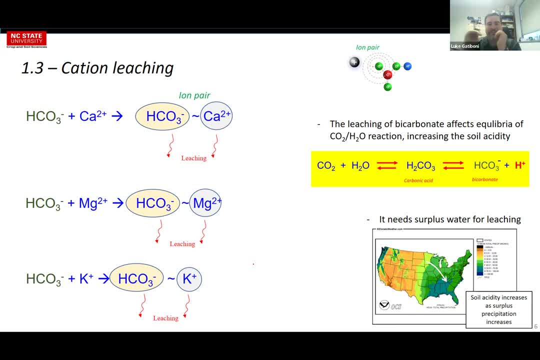 And why I consider this a cause of soil acidity. I consider this also a cause of soil acidity because when I am moving these biomes, when I am moving these biomes, when I am moving this bicarbonate from the soil, I'm decreasing the concentration of bicarbonate. 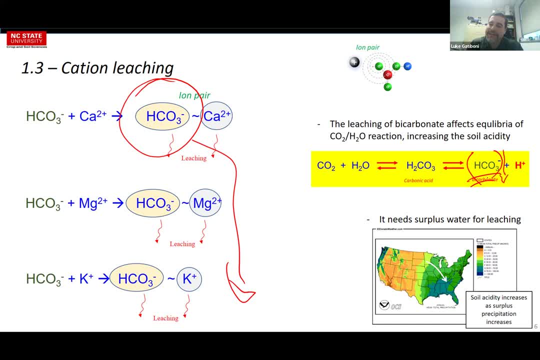 in the book solution. If I'm decreasing the concentration of bicarbonate in the book solution, this is a leisurely equilibrium And so if I'm decreasing the concentration of these products, I will increase the transformation of reagents in products. It means that I will move more carbonic acid. 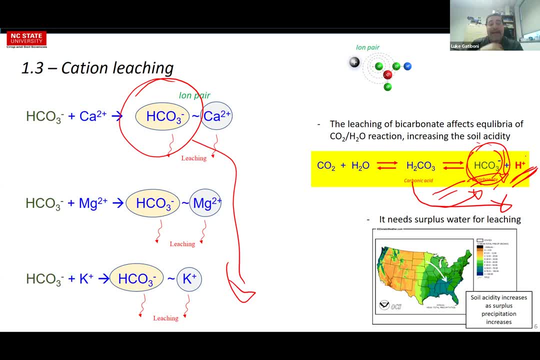 in this way and I'm releasing more hydrogen Again. it's not a big deal, but it's something that is occurring over the time and always when we have excess of water, I'm losing these basic cations and also I'm moving out of the profile some bicarbonate. 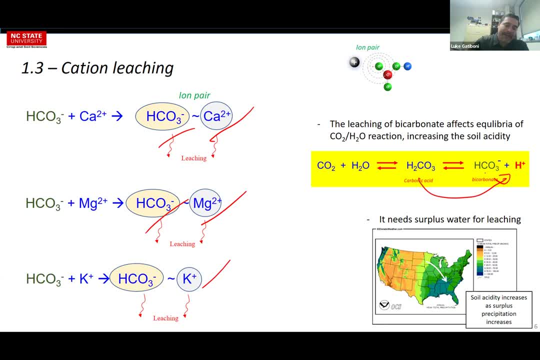 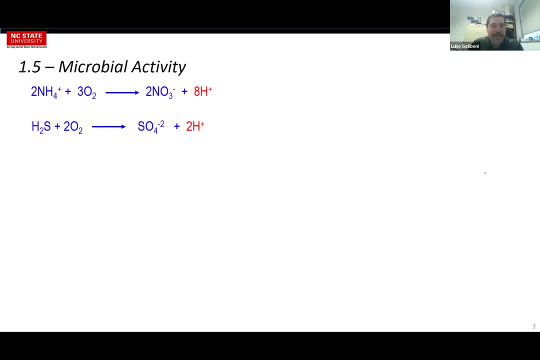 and this, in the end of the day, will increase a little bit the acidity, And so I have two bad things in this in this same reaction. The next thing that is a cause of soil acidity is the microbial activity, And we have a lot of transformations of nutrients in the soil. 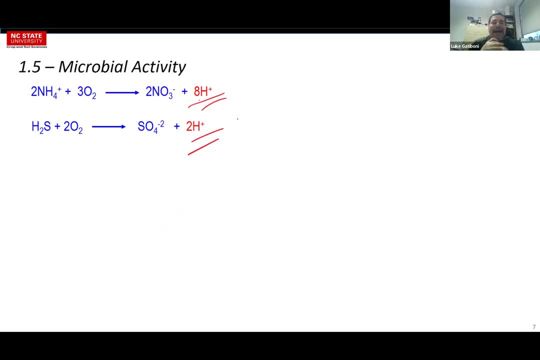 that we release during this process, hydrogen, And so the microbial activity- remember microbial activity. we have these transformations of nutrients, for example, but also have the microbial respiration releasing CO2, and CO2 will have that, that reaction that I just, I just showed you. 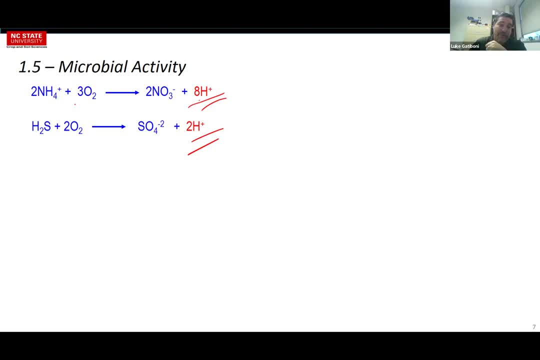 And one of the most important things related to microbial activity is the decomposition of soil organic matter, And when we have the decomposition of soil organic matter, we have the organic residues, and I'm looking here to an aerobic decomposition, and so I have oxygen. 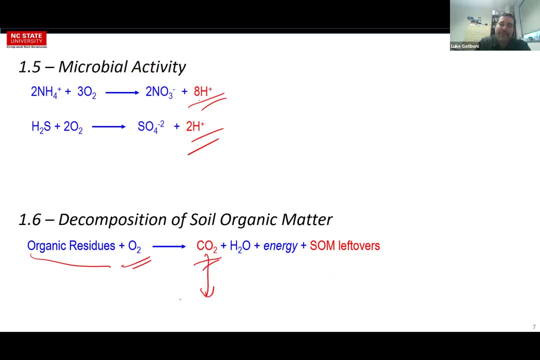 and I will release the CO2, and this CO2 can go to those reactions- 1.2, 1.3, 1.2 and 1.3- that we saw in the previous slides But also we have in the during the decomposition of the soil organic matter. 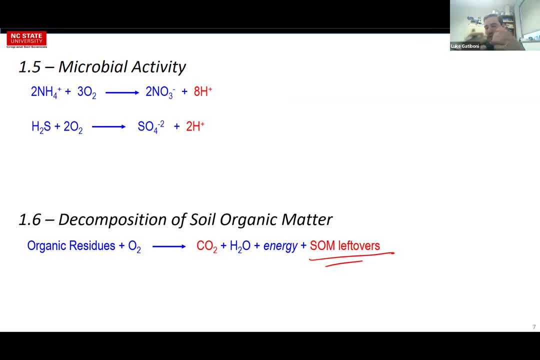 we have these chunks of carbon, chunks of material, organic material, that are leftovers that the microorganisms will not decompose. If the microorganisms decompose all the organic matter, the end reaction this CO2 and water, but it does not occur. 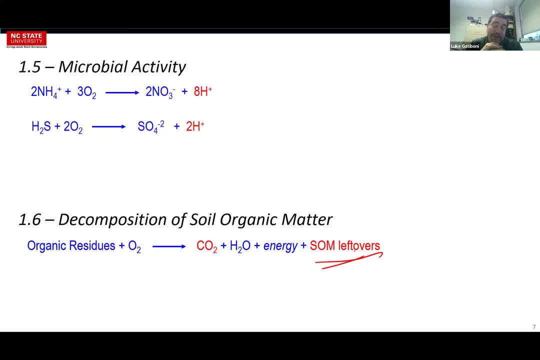 We have a lot of things that are released by the microorganisms because they not they cannot use all the organic matter, And so these chunks of organic material will being this: the soil will be our organic matter, or humus, or any other thing that you can name them. 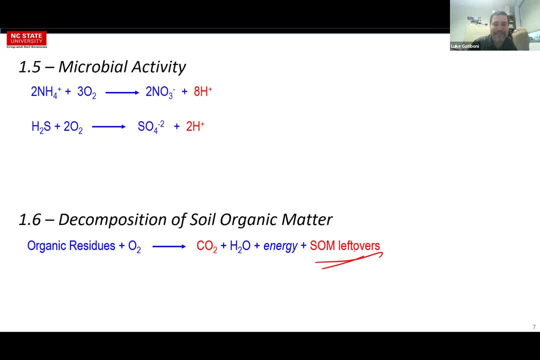 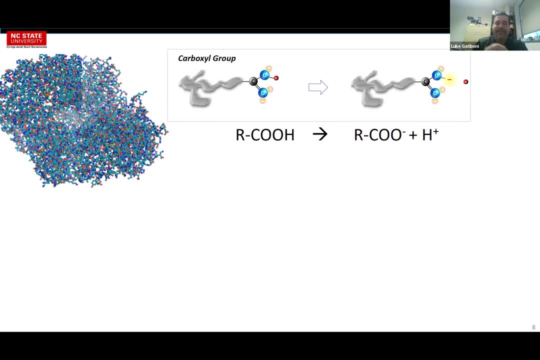 And how these leftovers affect the acidity. Well, we have different theories About how these organic materials react and in the soil, but we have these big organic molecules in the soil And these big organic molecules you have, we have in these molecules. 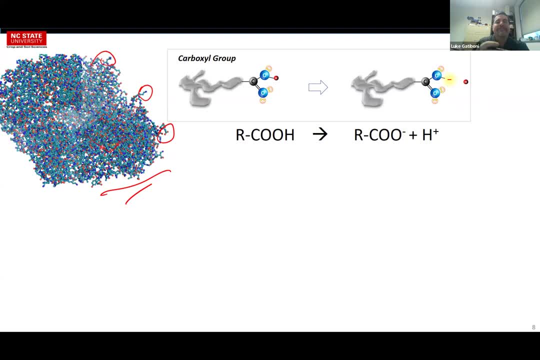 this end part, these radicals and these radicals. we have a lot of hydrogens that can be released from these radicals And I have an example here. This is a piece of organic matter and we have this carbon carboxyl group in the end. 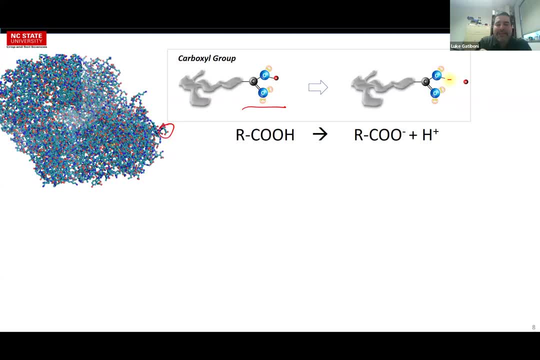 And I don't know, maybe this guy here and you can see carbon oxygen, oxygen. you have a hydrogen here And this hydrogen. we can detach this hydrogen from the organic matter and you can release it. We can buffer the acidity in this system. 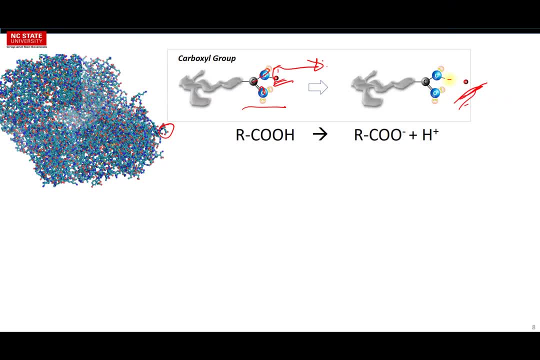 because it decomposes much, much more. Mike, get out of here What you doing, William, what do you have to do? Okay, We can see here the same reaction that we can see in the books: these radicals with these carboxyl ends. 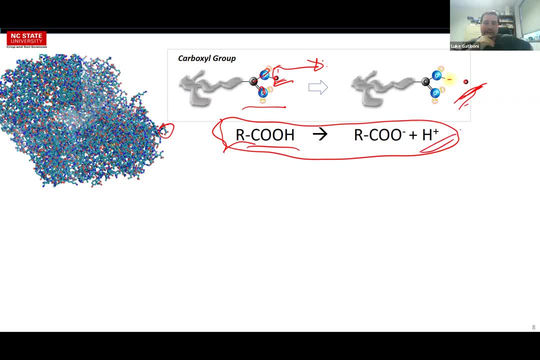 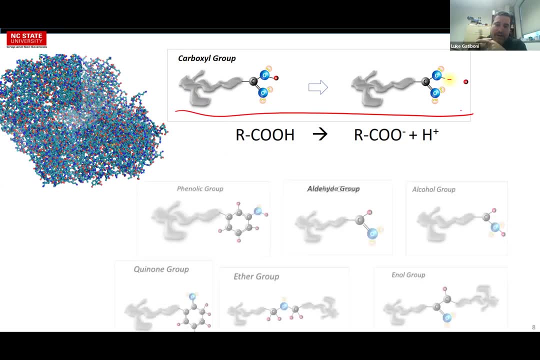 and we have here these hydrogen released from the carboxyl group. This is actually the same thing that I show in here, And this is not only carboxyl groups. We have a lot of different things in the organic matter that can release the hydrogens. 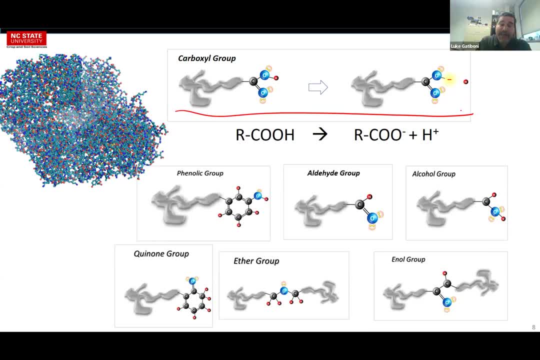 And we have here, for example, we have other radicals, but here we can have the phenolic radicals. and we have here, for example, we have other radicals, but here we can have the phenolic group: aldehyde, alcohol, quinone, ether, ethyl and many, many others. 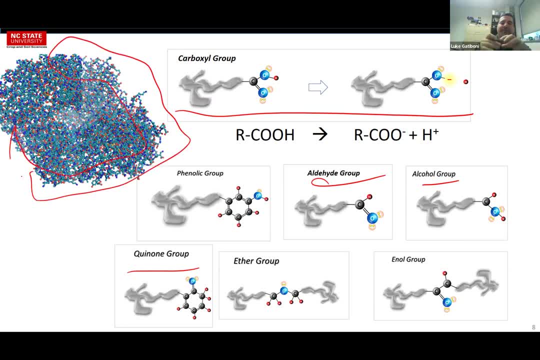 And all of these guys are buffering the acidity because these hydrogens can jump to the soil solution when we try to increase the pH applying line, for example- And it's important just to remember that the organic matter is formed from this hydrogen here. OK, 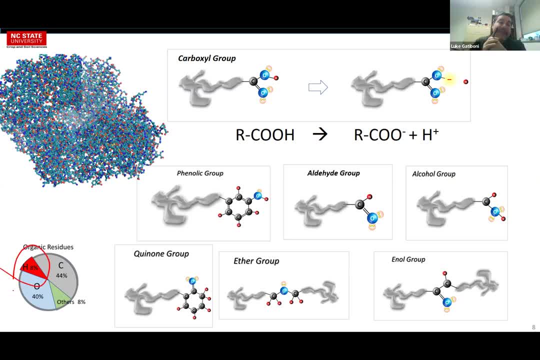 the organic residues, and we have about 8% of hydrogen in the organic residues, and so it's easy to understand why the organic matter do have this high capacity of buffering the acidity, because you have a lot of hydrogens in these materials, and so when you have more organic, 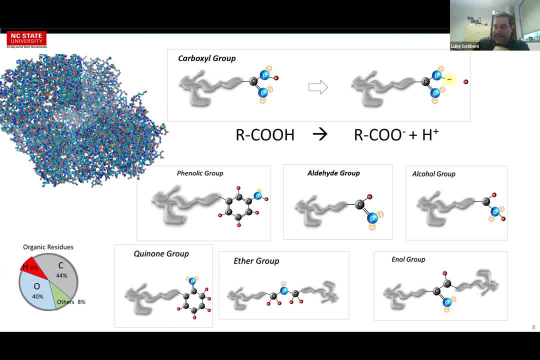 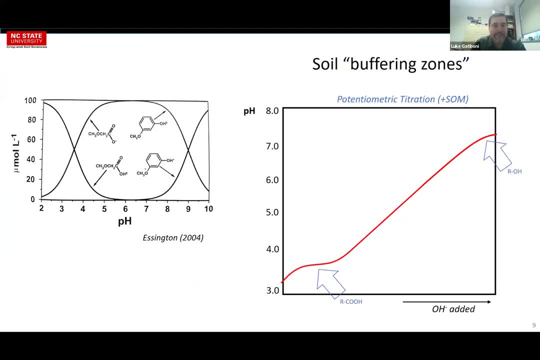 matter. we have more buffered capacity in this soil and because this is very hard to increase the pH of organic soils, for example- and here is an interesting thing about the how the organic American buffering the, the soil solution- we have these two very common groups, the carboxyl groups. 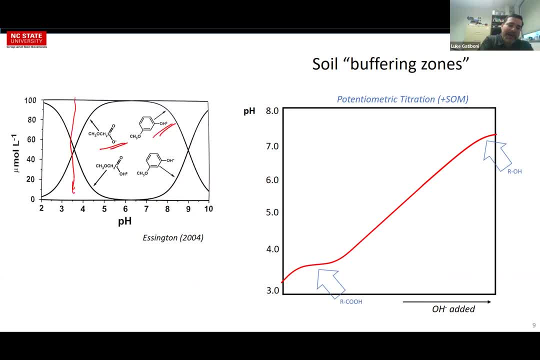 and the phenolic group and we have the pH where we have the release of these materials. for the carboxyl group, between three and four is the pH where we have the release of these hydrogens in the book solution and for the phenolic groups it starts after pH 7.. 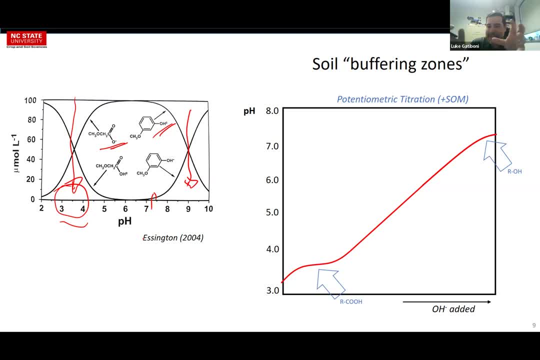 If you have a potential metric titration of a solution with some organic material and we have these two type of radicals there, we can see these deviations of our potential meth titration. Instead of being a one-to-one reaction, we have these parts where we need to apply a lot of hydroxils and we have this resistance. the pH will not. 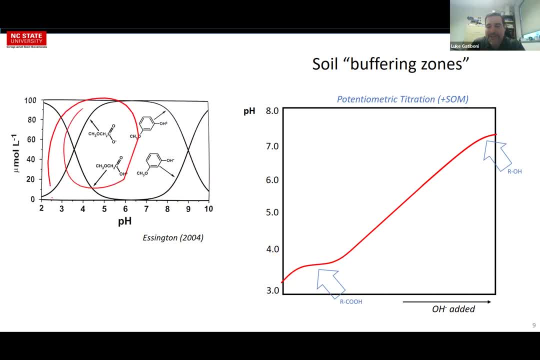 increase too much because you have the release of these materials in this part, in this area, in this pH zone, And so between three and four and four, we have some resistance to increase the pH when we are adding hydroxyls because you have this buffering capacity. 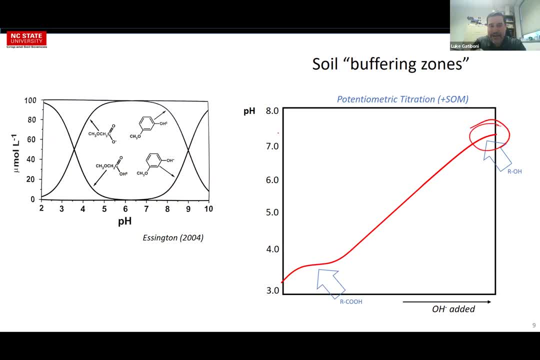 of the organic matter. We have another one zone here after seven because this. but when we think about our soil ranges, when we talk about agronomy, we are talking about maybe this range of soils for most of when we need to apply lime. 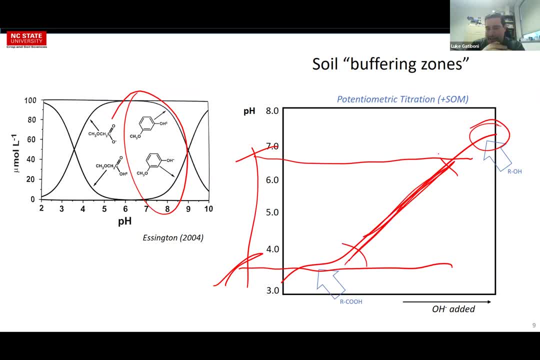 And so, for most of this part, we have this straight line of our potential metric deterioration of a soil. But it's an important zone to understand because you have resistance to increase the pH And because this is very hard to increase the pH of organic soils. 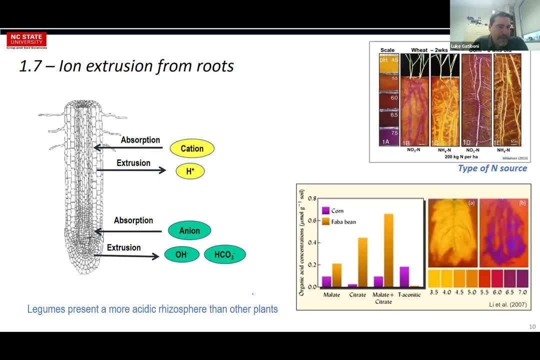 they are buffered at low pHs. Another cause of acidity is the ion extrusion from roots When we have a cation taken up by plants. if you have a positive charge here that the plant is taken up, the plant will release an hydrogen. 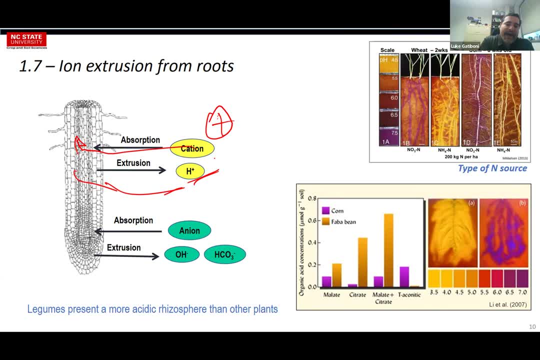 or another positive element, And for anion is the same. If the plant is taken up in nitrate, for example, it will release a bicarbonate, hydroxyl or an other organic material with a negative charge. The interesting thing is that when we have legumes, 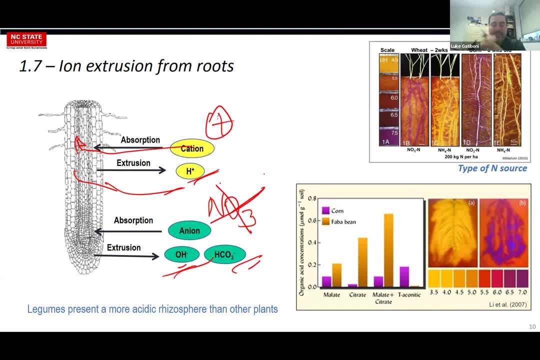 the legumes will not take up nitrate if they have the biological station of nitrogen. And so for legumes it's as they do not take up anions too much as other plants. they do not release a lot of hydroxyls or bicarbonate. 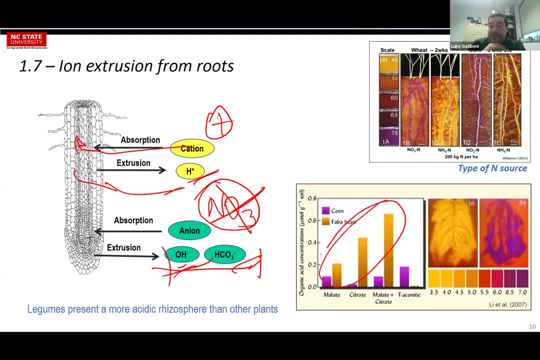 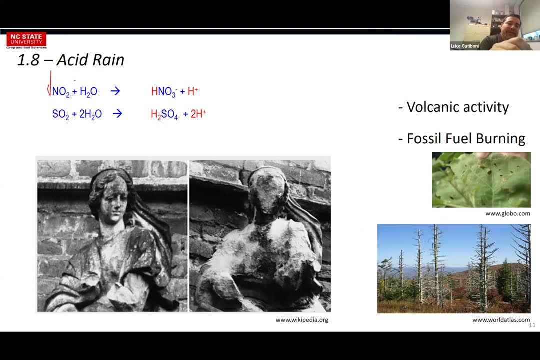 And so it's common to have acidic rhizospheres for legumes, and it's another component, another cause of soil acidification. Another component is as the rain, and as the rain will occurs when we have components- nitrogen and sulfur components- in the atmosphere. 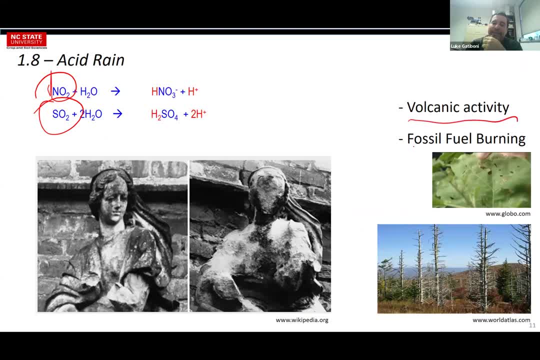 relates especially to volcanic activity or fossil fuel burning pollution, air pollution in general, And these will generate acid rain. and we have- we can burn plants or we can have these ghost forests. Ghost forests can be provoked by acid rain or also by salty soils, for example. 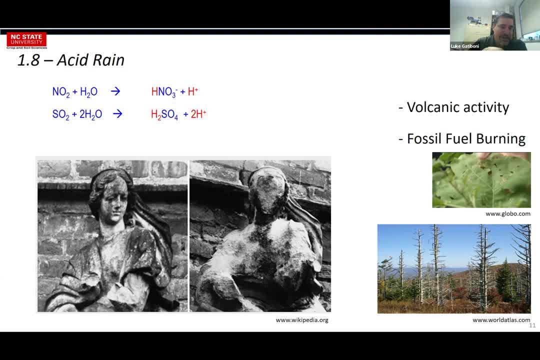 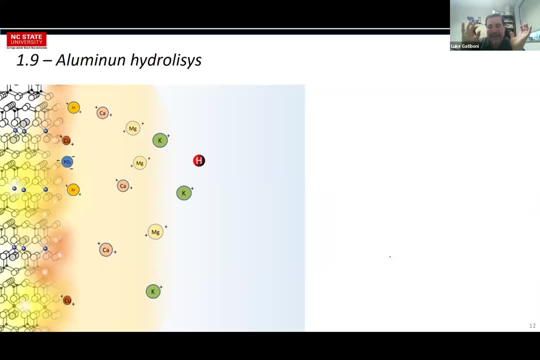 And this is another cause of acidification. And we have only two, the last two And for me is the most important two, And now I will talk about the cracking. the cracking of soil acidity is the aluminum hydrolysis And the hydrolysis of aluminum. 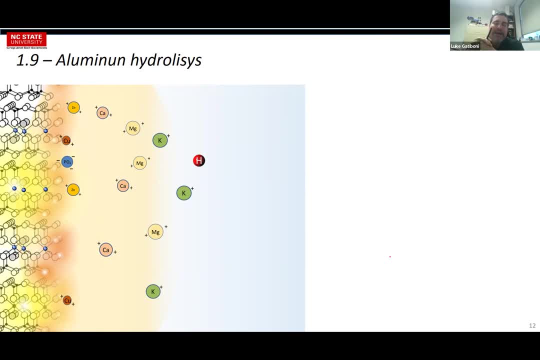 it's a very important cause, especially when we have a very low pH. When the pH is below 5.5, we start to have these aluminum hydrolysis And I show you how it works. We have hydrogens in the book solution. 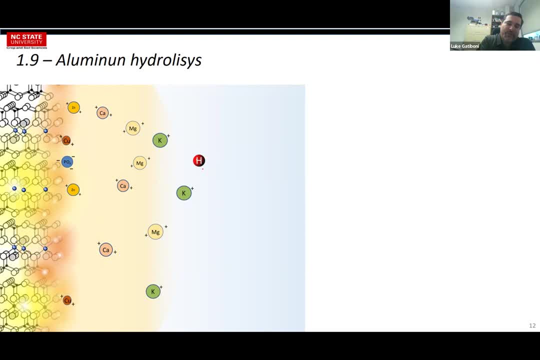 and these hydrogens, because hydrogens are very- it's just a proton. a proton, sorry, It's a very small cation, This hydrogen, when you increase the concentration, or it means when the pH start to drop, these hydrogens will start to move to the CEC. 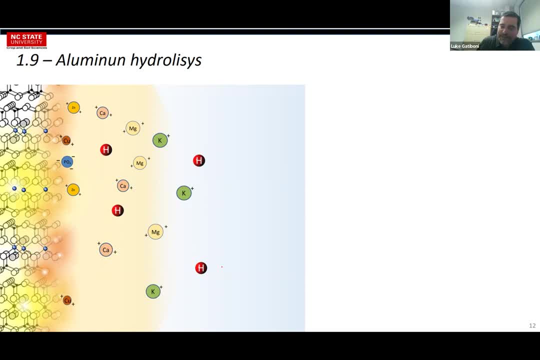 will be attracted by the charge, the negative charge, And they will start to populate this part of our clays, in the edge of the clays, because hydrogens are very is very small And so they can just move very fast and attach to the soil particles. 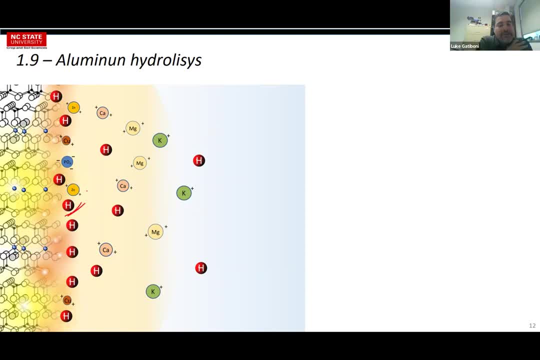 The problem is that the hydrogen. hydrogen does not stop in this edge of the clays Because hydrogen is very small. hydrogen just start to invade the clays, especially starting in the interlayer of two to one. So it's very, very small. 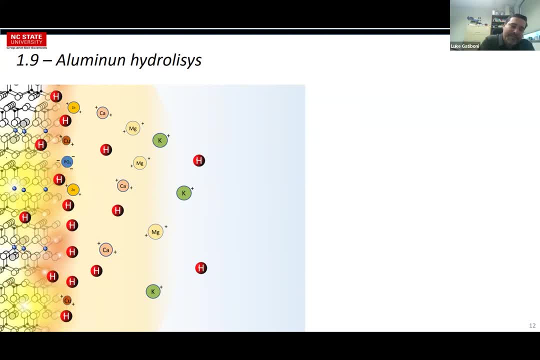 And if you have two, one clays and, but it will also force in other type of clays And the hydrogens start to invade the the inside part of our clays and in the inside part of our clays. 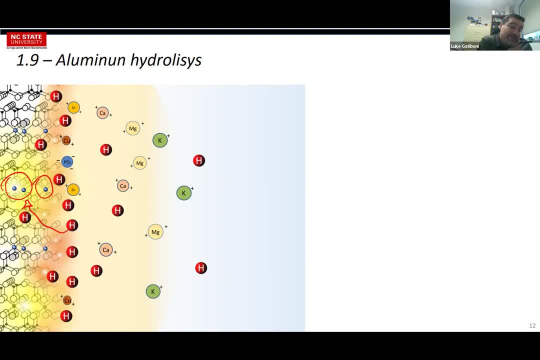 you have aluminum in the octahedrons of those clays And when the hydrogens start to to degrade these clays, we start to push aluminum, We start to push aluminum, We start to push aluminum, Aluminum to the bulk solution. 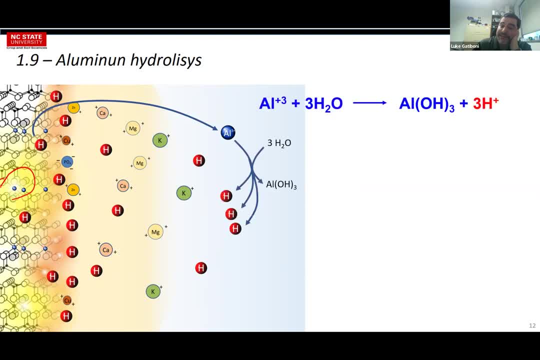 And aluminum in the bulk solution will have this reaction. Aluminum in the bulk solution will react to water and will precipitate aluminum as an hydroxide, And I will release three hydrogens for each aluminum that I have, And so this is the bad thing about aluminum. 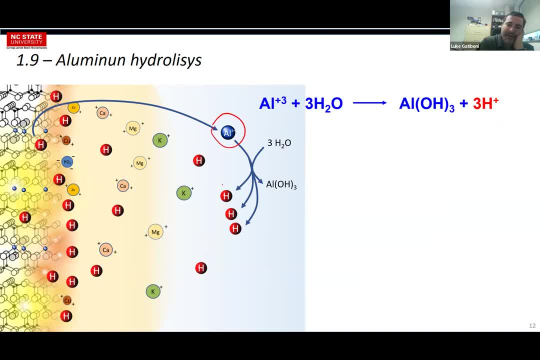 because when aluminum comes to the bulk solution, aluminum will release a lot, of, a lot of acidity And this acidity will go back to the clay and will release more hydrogens, more aluminum, sorry, And we start to have this process that is increasing a lot the acidity. 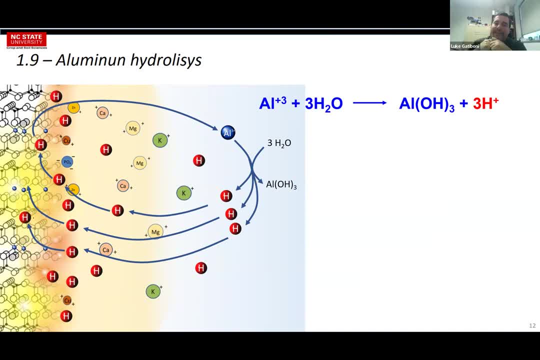 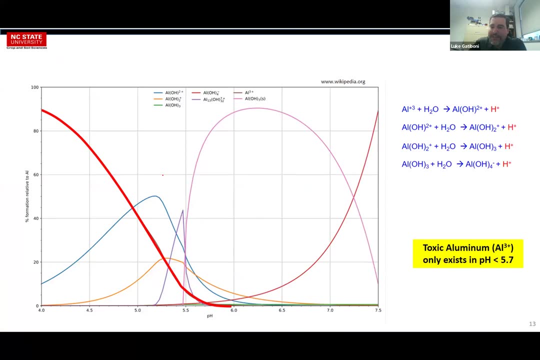 And so when we start to release the aluminum in the bulk solution, the acidity will increase very fast. reaction of aluminum in the bulk solution: And you can see here this is the equilibrium of the different forms of aluminum in water And you can see that all of these transformations. 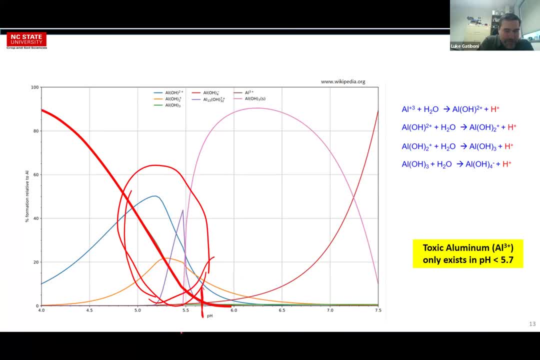 will occur in pHs below 5.7,, but especially in this range of 5 up to 5.5,. in this range of pH we have a lot of transformations. These forms of aluminum will start to occur, And so when we 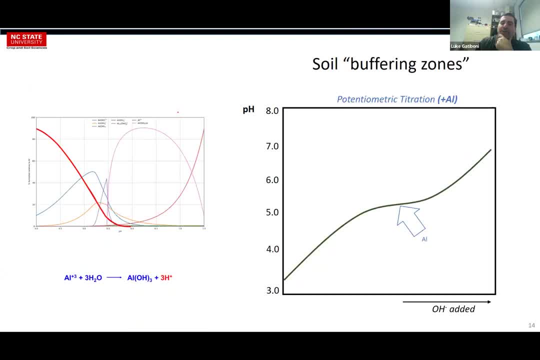 think about the soil with aluminum. we have another buffering zone in soils in this range between 5 and 5.5.. It means that if I'm starting to add hydroxyl in my soil or I'm using lime, for example, we have another buffering zone in this range between 5 and 5.5.. It means that if I'm starting to add hydroxyl in my soil or I'm using lime, for example. we have another buffering zone in this range, between 5 and 5.5.. It means that if I'm starting to add hydroxyl in my soil or I'm using lime, 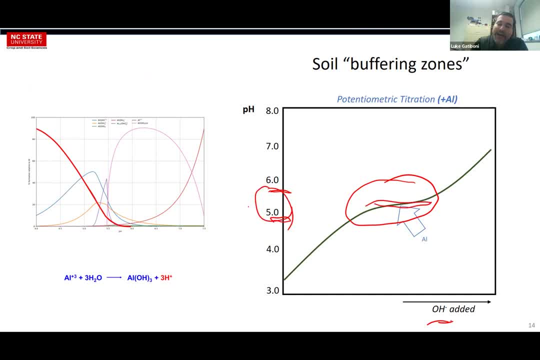 it means that if I'm starting to add hydroxyl in my soil or I'm using lime, we have a resistance to increase the pH when we are in this range of 5 to 5.5, because we have a lot of things going on. 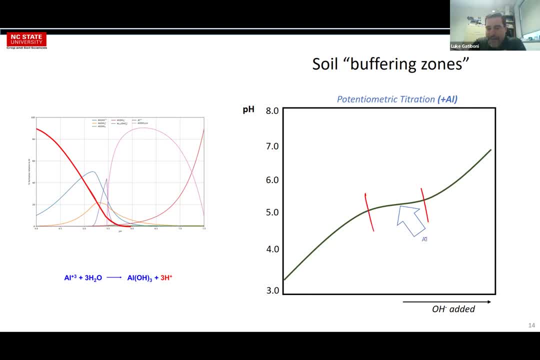 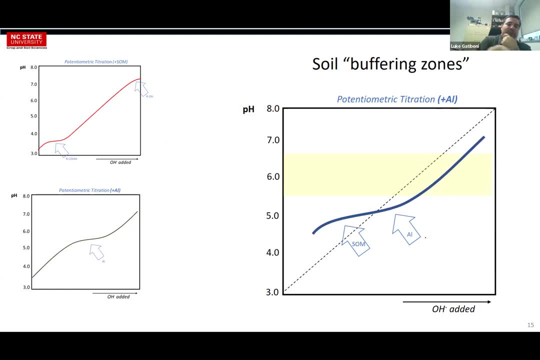 with aluminum in this pH range, And so this is another thing related to aluminum. And so when you think about the organic matter, remember that we have the organic matter buffering at low pH, then we have the aluminum buffering at low pH, then we have the aluminum buffering at 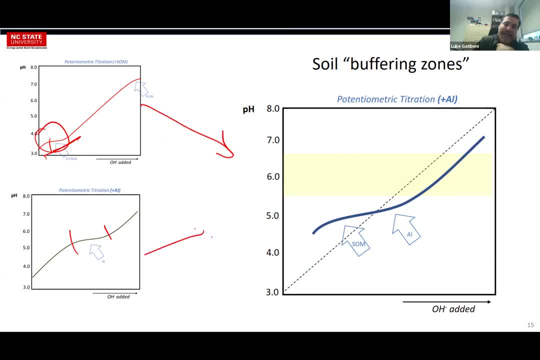 5, 5.5.. When you put these two things together in only one graph, we can see that we have this part that is predictable, that it's the equation. we can use a linear equation to predict the amount of lime or hydroxyl that I need to neutralize acidity, But when I'm 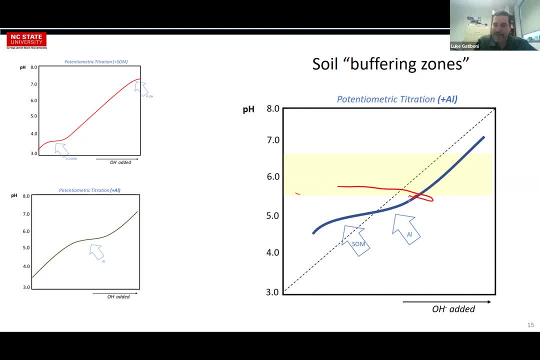 adding the plastic and when I'm adding these. But when I'm adding the plastic and when I'm adding these two things, you also see that I have the pH below 5.5, we have this deviation because you have this buffering capacity of the soil And so when we are in this area, we need to apply. 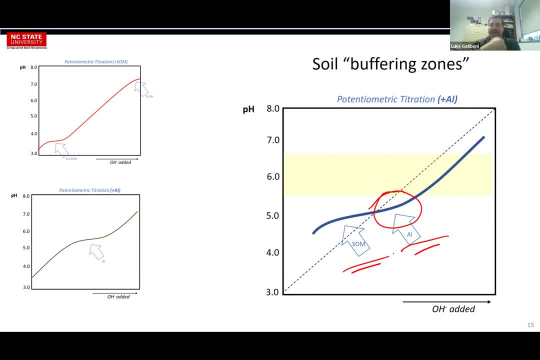 more lime, because you have the buffering of aluminum and the organic matter in these low pHs And I remember from our last presentation Frank showed that we need to. I think it was buffering from the Schumacher dissertation. I think that exactly this region where we have 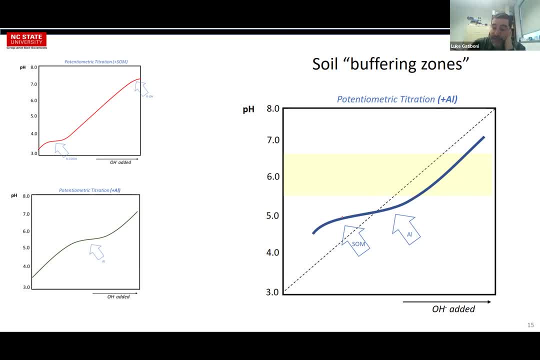 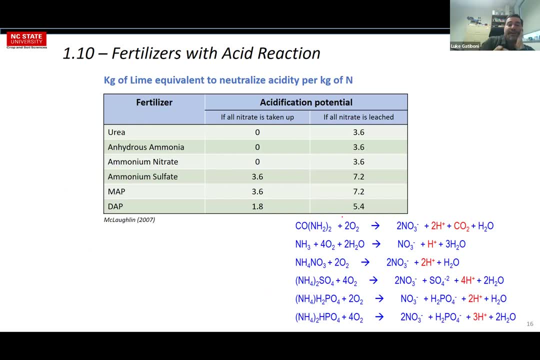 aluminum, buffering our pH. It's a very interesting thing. And the last cause of acidification is the fertilizer with the acid reaction, And so I told you that the last two are the worst causes of acidification. The first one is aluminum in the last, and the second one that is very hard is the 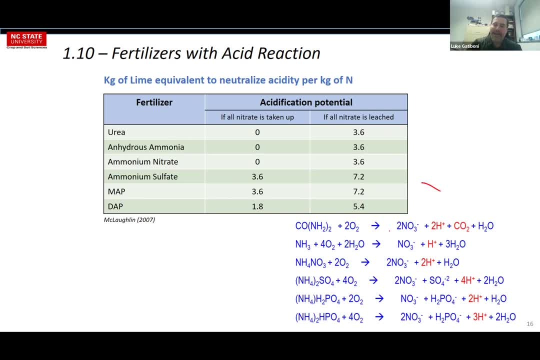 fertilizer, especially nitrogen fertilizer, We have this capacity of releasing hydrogen, And when we think about agriculture in the United States, where I don't think we have the most of our soils, we use lime in a regular base, And so aluminum is not a problem in most of the cases, And so this is the 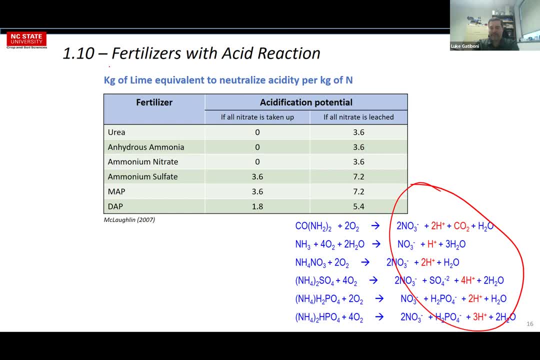 biggest cause of acidification. The second cause of acidification in our soils, the use of fertilizers. I'm coming from a different mindset. I'm coming from a tropical soil, a tropical region, And for us aluminum is the worst problem. All our soil reports. we have exchangeable aluminum in the results, because 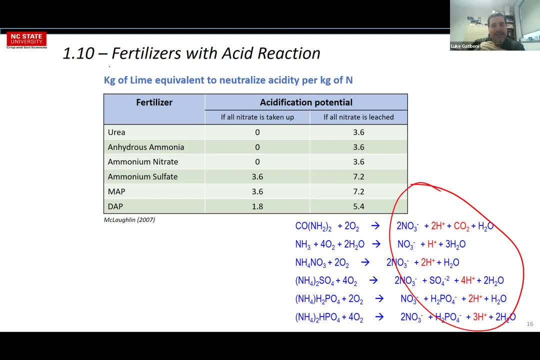 they are very common to have dislocates And so it's an important thing for us When you come from. for example, when I came to North Carolina and I look at soil test report, where is aluminum? You don't have because you have pHs in general, except for organic soils. 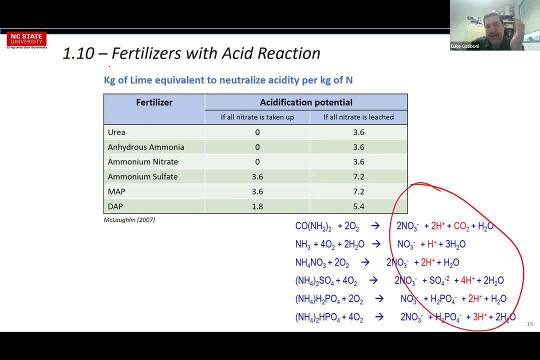 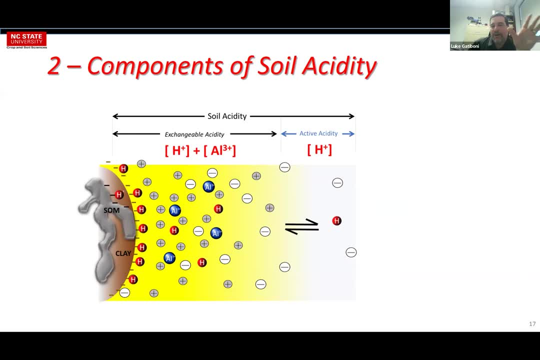 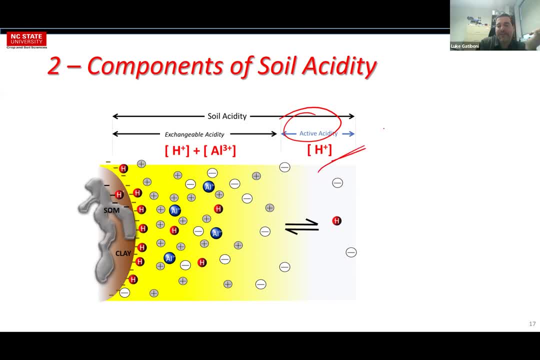 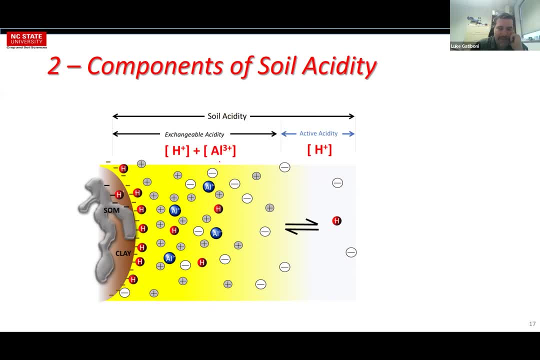 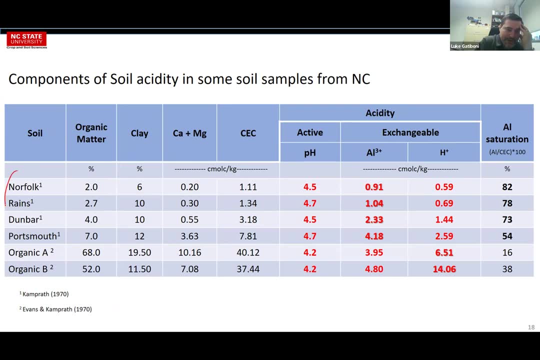 aluminum in the CEC, depending on the pH that we have in our system, And we can see here some North Carolina soils. We have here some soils that are mineral soils and organic soils. We can see that in mineral soils aluminum is. 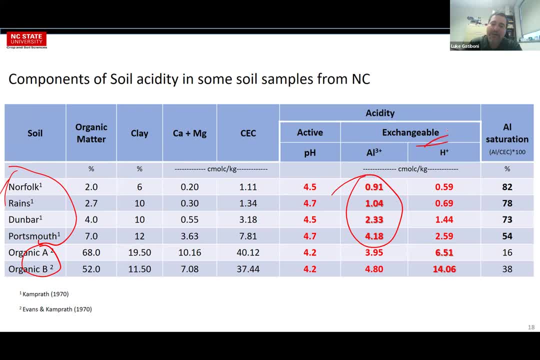 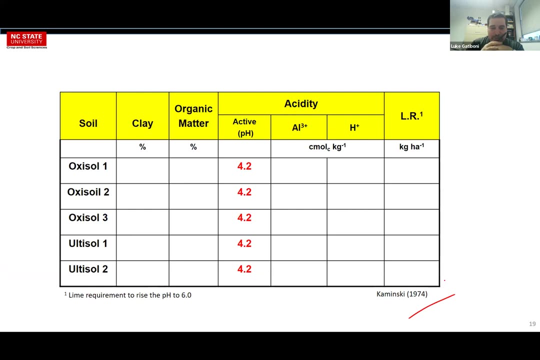 is a main component of the exchangeable acidity, while in organic soils the hydrogen from the organic matter is the main component of the acidity And this is some results from tropical soils And I like to show this just to debunk some problems with the activity acidity. 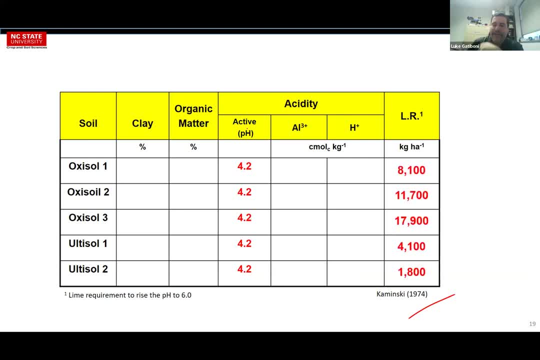 I have here five soils with the same pH but with very different limey requirements, from 1.8 metric tons per hectare up to 18 tons. And what is driving this? What is driving this is the amount of aluminum and the amount of hydrogen that we have in these soils. 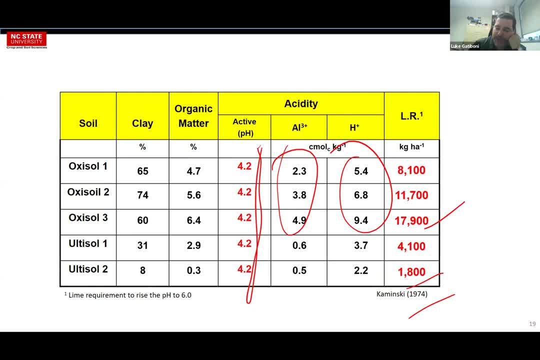 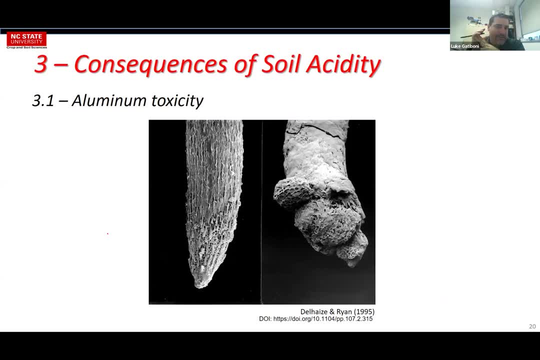 even with the same pH, they have a very different exchangeable acidity. Okay, the last part is consequences of soil acidity And the first consequence, of course, if you have a pH below 5.5, is the aluminum toxicity And you can see the deformation. 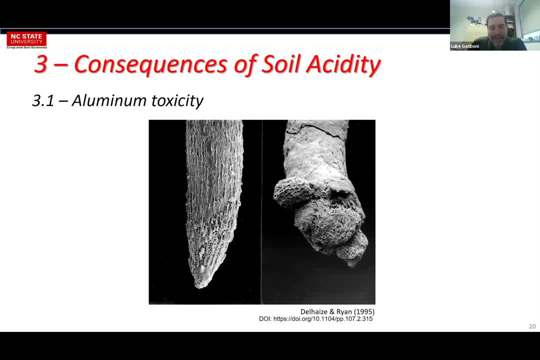 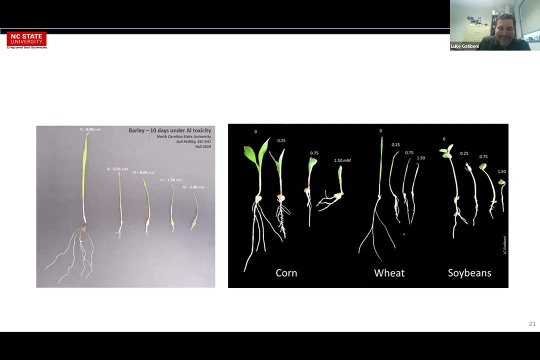 the monstrosity that we can produce when we have aluminum. in the book solution, Here is a healthy root and here is a non-aluminum root And here is a root of aluminum And I always show to my students in soil fertility. 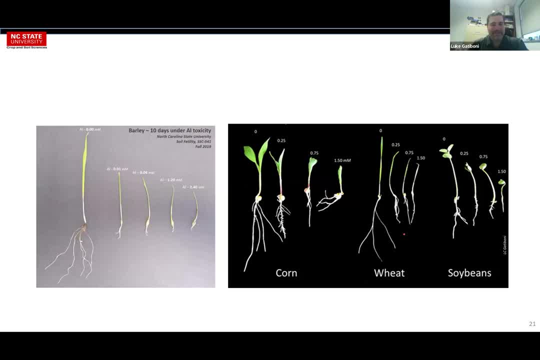 I make these with solutions of different concentration of aluminum And I show them just to scare them about acidification and the effects on, for example, in barley corn wheat, soybeans. every semester I do the different plants to show them this effect. 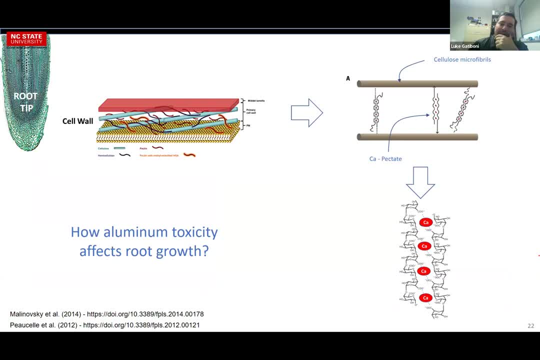 And what is the problem with aluminum? The problem is that we have in the microfibrils, in the cell walls, we have these calcium grids. that makes all these things together in the cell wall and the aluminum will replace the calcium here in these spots, and we started. 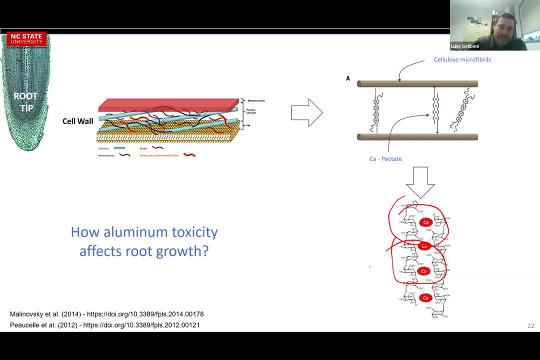 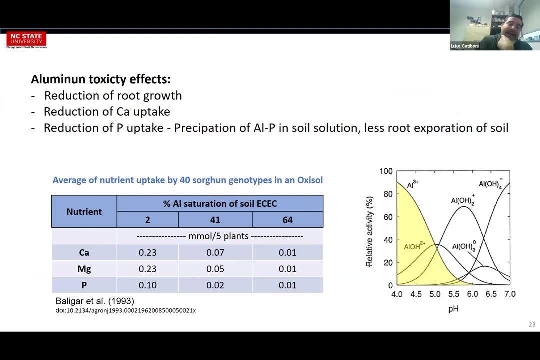 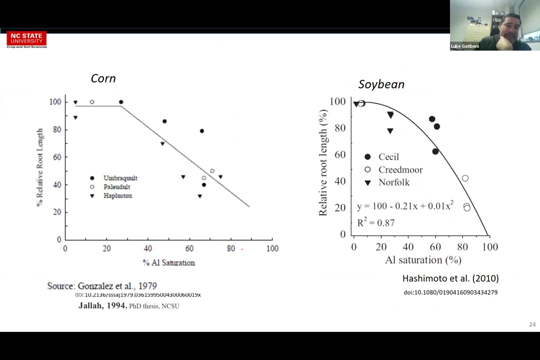 to have the deformation of the cell walls because aluminum is the replacing calcium And we can see that when we have higher aluminum saturation in the soil we start to drop the nutrient uptake because the roots are not functioning in the right way. And we can see here some examples of aluminum saturation in the soil and the effect on corn and soybean. 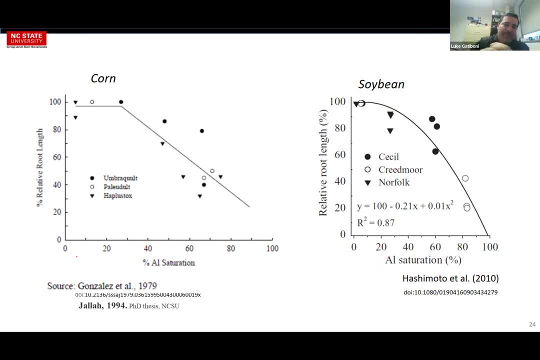 And for different plants you have different thresholds. For example, for corn and soybean the threshold would be between 15% and 30% depending on the variety, But we can have some plants, like barley, that cannot have more than 5% of aluminum saturation. 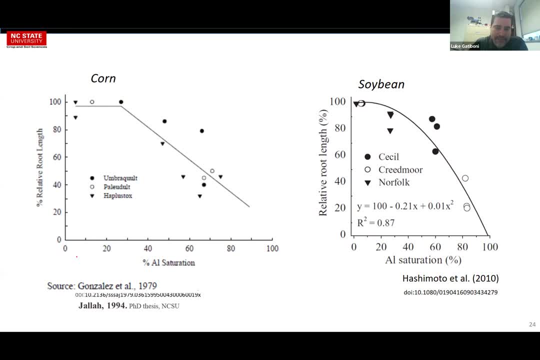 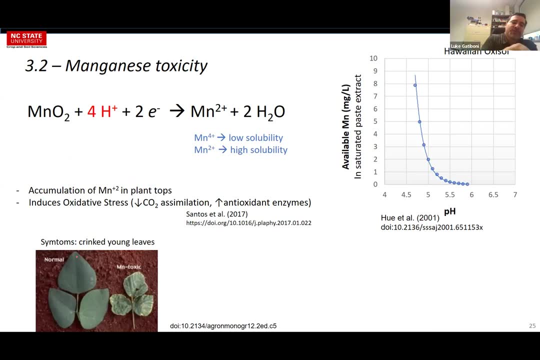 Because they are very sensitive And also cotton is very sensitive. The other problem that we can have is manganese toxicity, And manganese toxicity will occur because in low pH I can dissolve the manganese oxides on the soil And I need acidity for that And we need some electrons. It means that we need some reduction in the soil. 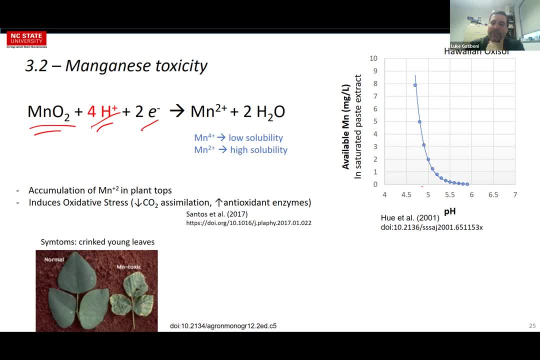 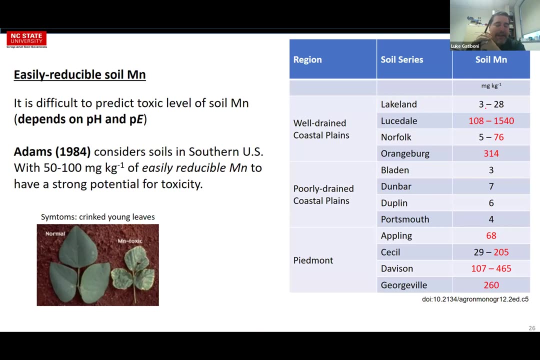 And the problem with manganese toxicity will occur At very low pHs- below 5, below 4 most of the time. But it depends on the soil, because you need to have manganese oxides in your mineralogy, Otherwise you don't have manganese problems. 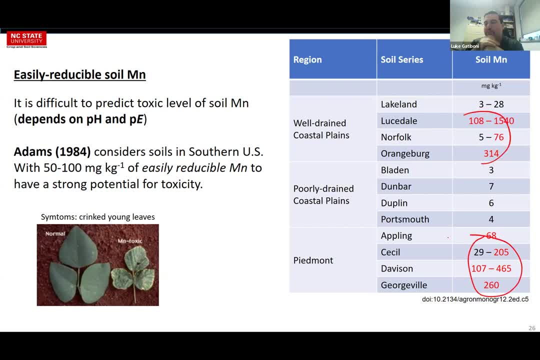 And so here are some soils for North Carolina. You can see some soils that will have more manganese oxides, minerals of manganese, And so in these soils, if you have a very low pH And you have some reduction potential in the soil, manganese could be a problem because of the toxicity. 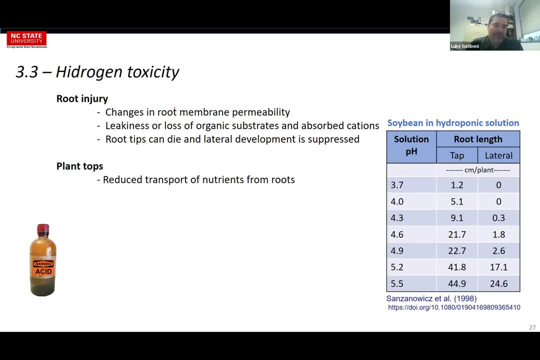 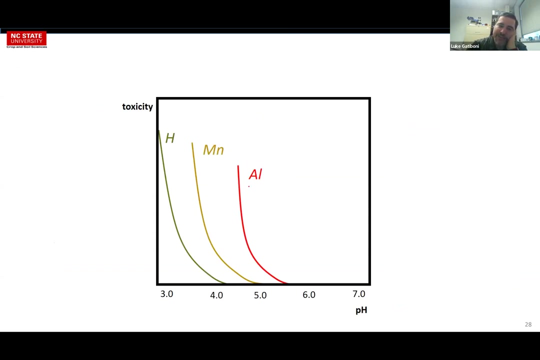 The other problem is hydrogen toxicity, And hydrogen toxicity is just because hydrogen will dissolve the roots And in very low pHs we start to have problems because the hydrogen dissolving the tip of your root hairs. And when you put on All these guys in the same graph, we imagine that the aluminum is the first problem. 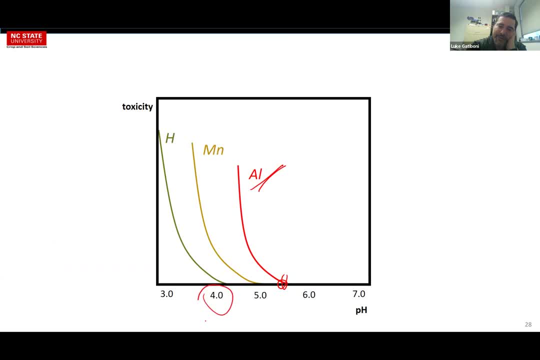 We will start at 5.5.. Manganese will start about pH 4 and hydrogen problems will start at very low pHs like 3 or less, And of course all of these depend on the plant species. Some species can hold very low pHs without any problem. 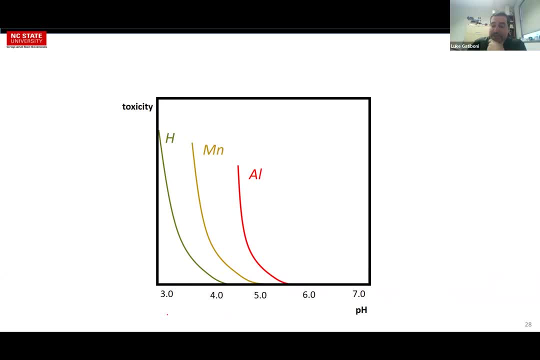 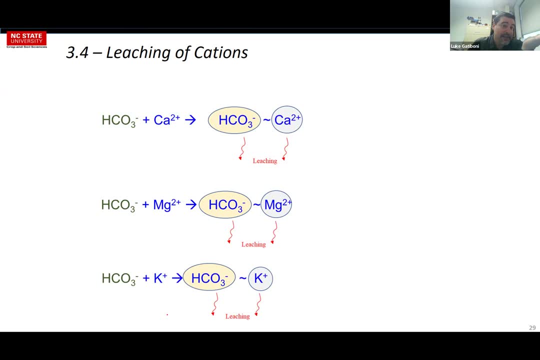 So it depends on the tolerance of each plant to these toxicity problems. The next problem that we have with acidity is the leaching of cations, And remember, it's exactly the same thing that I showed you as a cause of acidity And now I'm just putting here as a bad consequence, because I'm leaching essential nutrients when you have acidification of the soil because it's leaching. 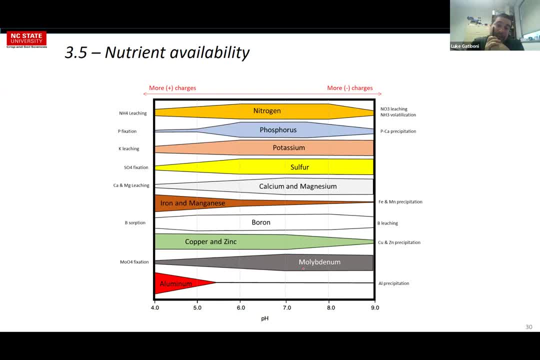 And the next one is nutrient availability, And I'm sure all of you remember This figure. when we have different pHs, this range of pH, we have problems in the ends of these. for example, for nitrogen, we can have leaching of ammonium or it can have lifting up nitrate in high pH, and phosphorus will have fixation low pH. we have precipitation of calcium in high pH, and so on. 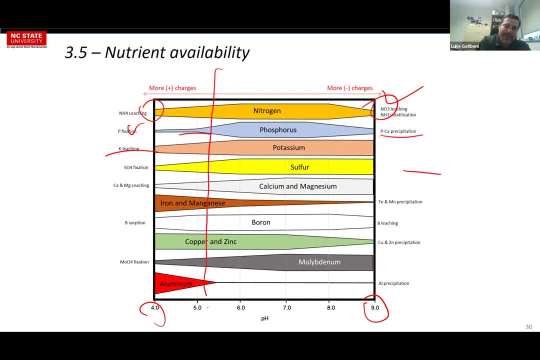 It means that we have a range of pH here that we have less problems and problems. Okay, Okay, Okay, Okay. So this is the good range for our plants. Remember, we don't want to have aluminum, so our threshold will be some like here: until here would be a good range of pH. 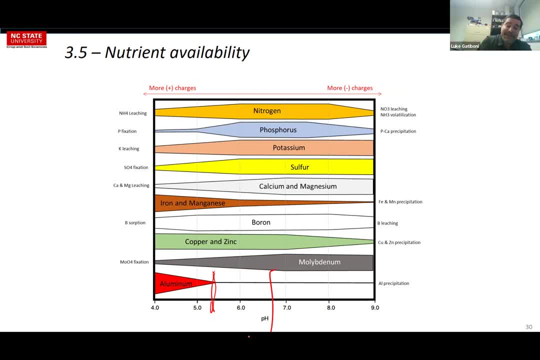 Of course, for organic soils we don't need to have a pH higher than 5.5, because in organic soils we don't have too much aluminum. We have a lot of organic materials as the materials that are the solid components, And so it's not a big deal for organic soils, and a lot of aluminum are also complexed by the organic materials in our organic soil, and so aluminum is not freeing the solution in organic soil. 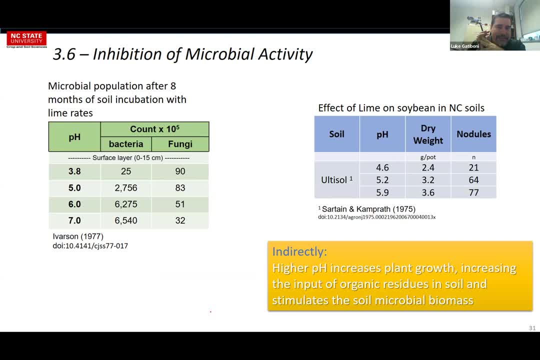 And the last cause of our acidification is the inhibition of microbial activity and you can see, when we have very low pH, we are decreasing our pH. decrease in the especially bacteria activity in the soil, and this is not good. decrease in the especially bacteria activity in the soil, and this is is not good. 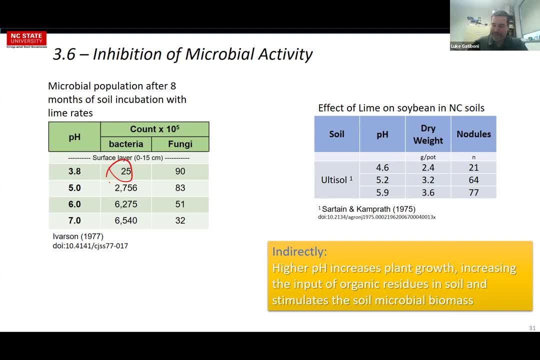 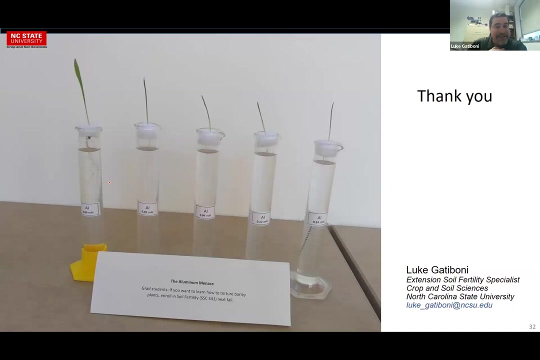 when you think about the how the microorganism can can help the soil function in a right way, thinking about cycle nutrients, transforming nitrogen and processing organic materials in the soil, and so And that's it. this is the causes, the components and the consequences of the soil acidity. 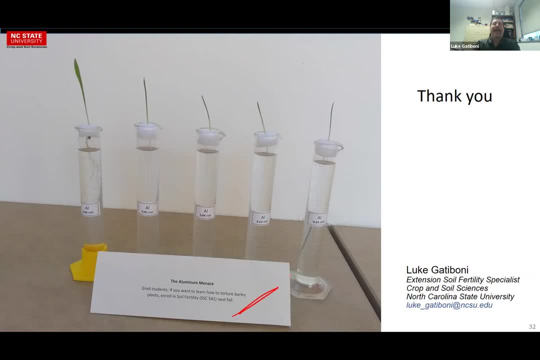 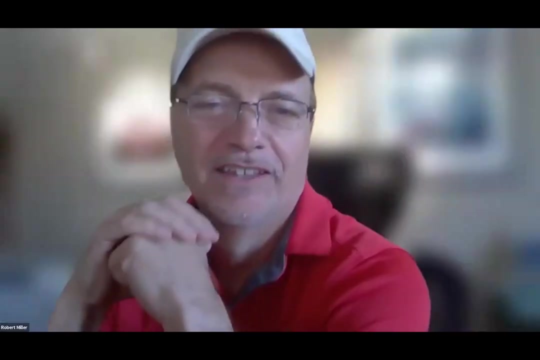 This is. I put some semesters in the hallway of my department to attract some students to soil fertility, and my advertising is how to torture plants with aluminum. And so that's it. that's my presentation, Bob, Thank you. thank you very much, Luke. Let's have some questions out there. I mean, I really appreciate the detail that you went into this on and I have some questions, but I'm going to throw it out to the rest of the group first, So go ahead, anybody questions? 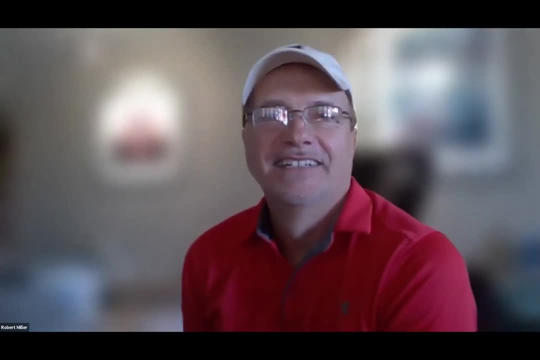 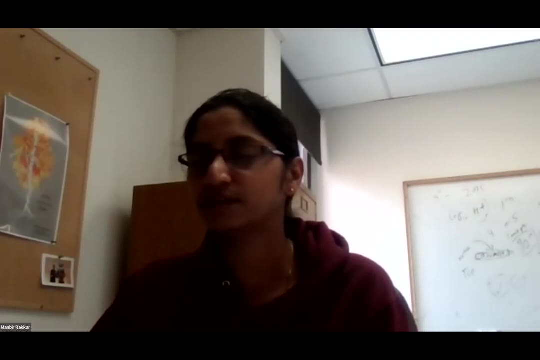 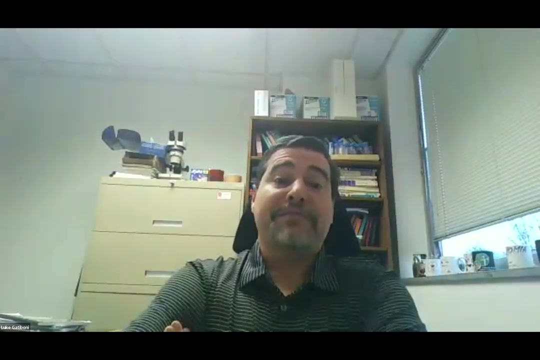 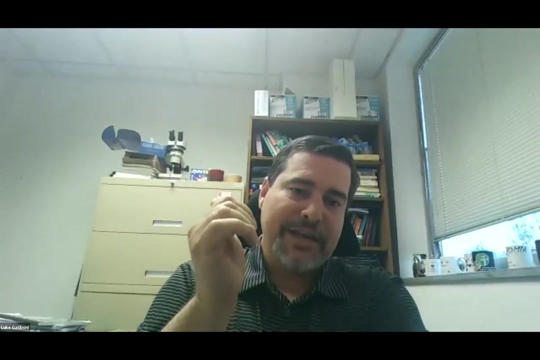 Hey Luke, this is Manbir. Just wondering. when we talk about legumes, is it the aluminum toxicity or is it the locus, Or is it the low pH that affects the rhizobium? We have both things. in general, the legumes will have this rhizosphere with low pH. And it depends on how low is the pH. if the pH is lower than 5.5, we will have both problems. We will have the low pH in the rhizosphere and at the same time, we'll have the aluminum problem in the rhizosphere because the pH is very low. 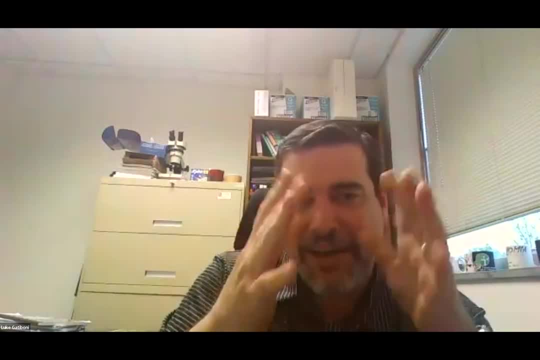 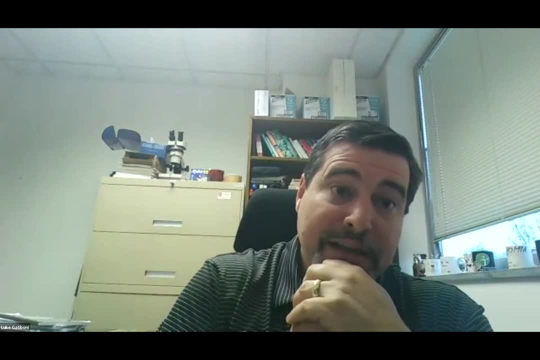 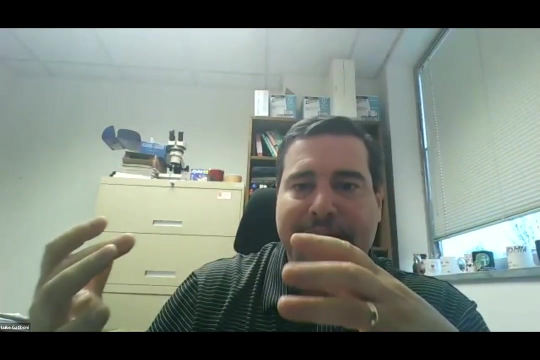 But in general we have that very thin layer Of soil around the roots that we have this low pH And of course it depends on the plant. We have some legumes that can hold this acidification of the rhizosphere very good, because they can release some organic materials and ions that can complex this aluminum. So aluminum is there, but it's not free for the plant taking up And it causes problems in the roots, And so it's just a general thing. in general, legumes are more sensitive to acidification. 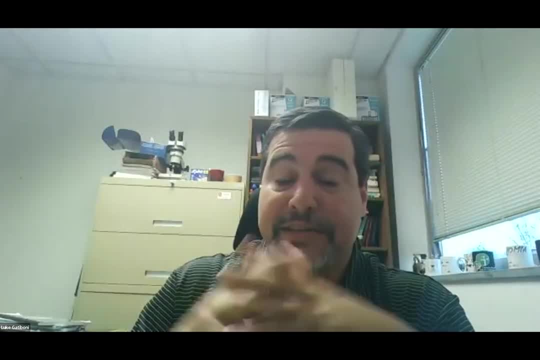 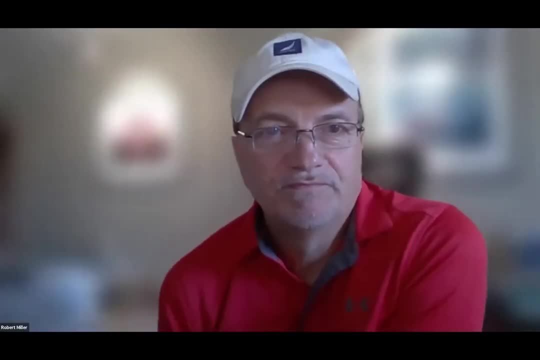 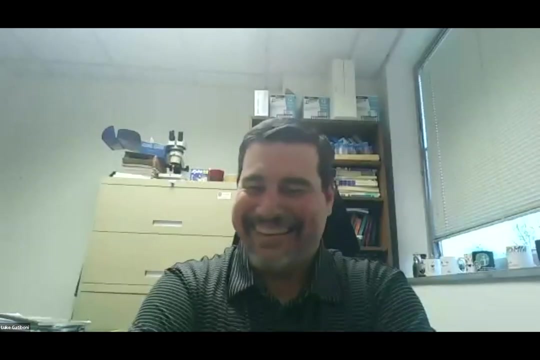 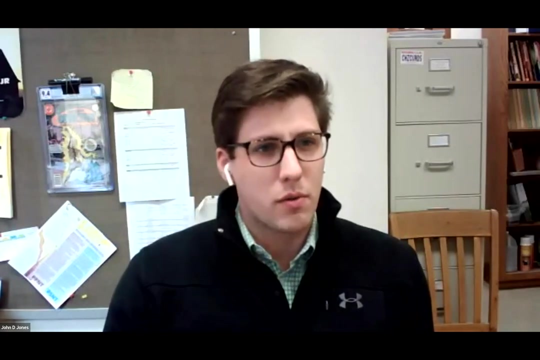 than grasses, just because this is the acidity in the rhizosphere. More questions. Wow, everybody's quiet today. Go ahead, John. Yeah, I have a quick question. I just had kind of an extension type question. I had an extension type conversation with a grower in the Central Sands region of Wisconsin. Very coarse soils, a lot of potatoes, vegetable crops and we had a conversation about potassium leaching And we always see, you know, non acidic cations as a source and result of low pH environments. Have you seen any estimates on actual pounds per acre of leaching of some of these cations? 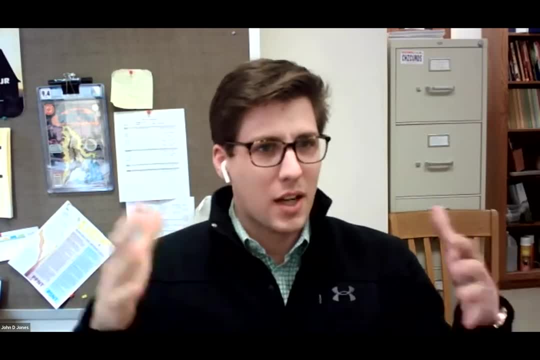 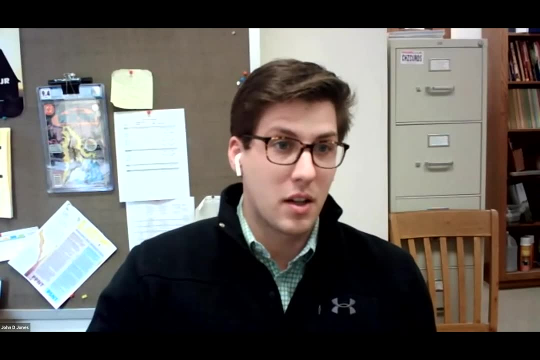 I'd be really interested to see some numbers on that, sometimes Because we just kind of throw it out there that this process leads to this, But it'd be interesting to put some numbers, because we don't have data on K leaching. honestly, 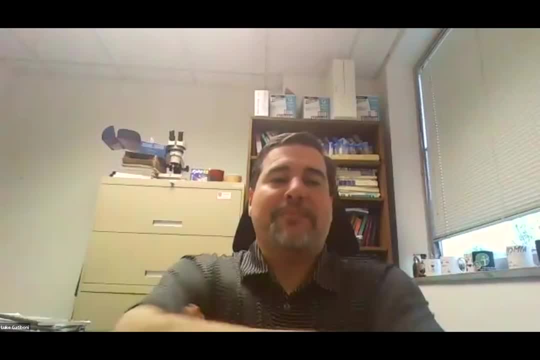 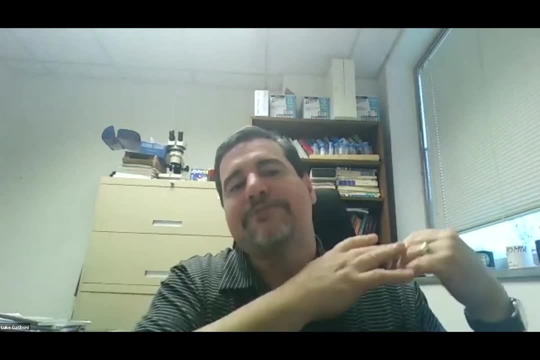 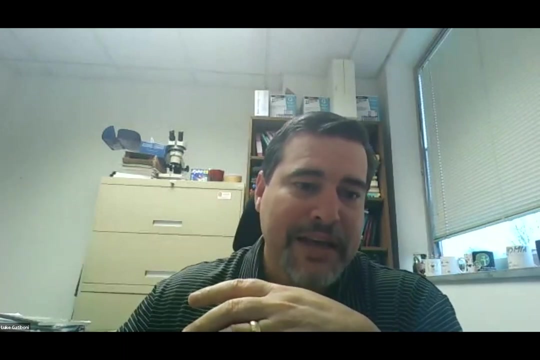 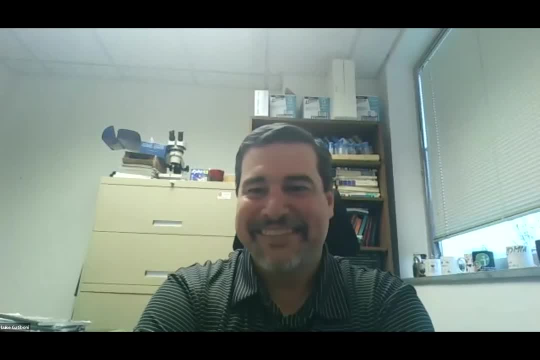 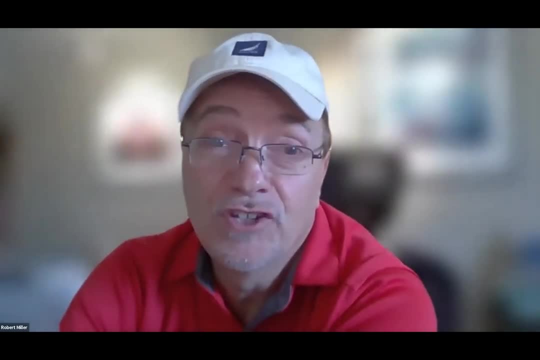 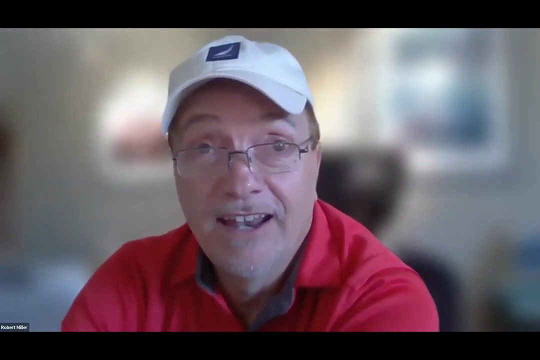 So, John, I'll make one more additional comment along the same lines, being that you're talking about potatoes and the high nitrogen usage that they put into those crops and therefore the high potential for anemone nitrogen you know to be breaking down into nitrate and therefore all the hydrogen release. it could be a big deal. 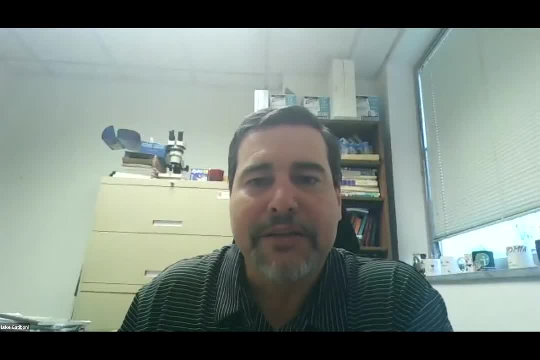 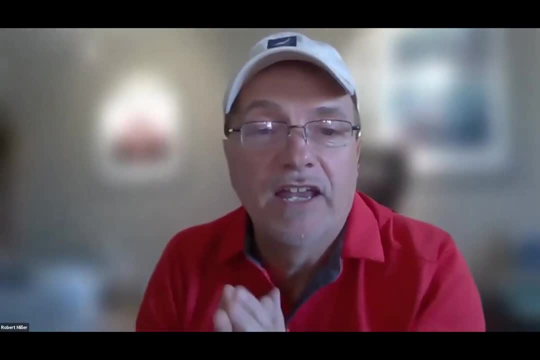 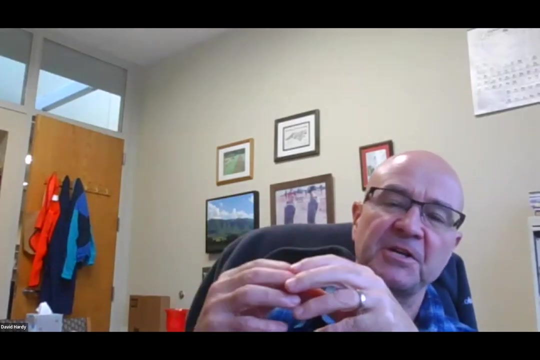 I think Dave wanted to add something Not related to that, but on leaching. but you go ahead. No, no, that was all. I'm just making a comment. Go ahead, David. The thing you mentioned leaching, about bicarbonate being the companion anion with leaching of bases. 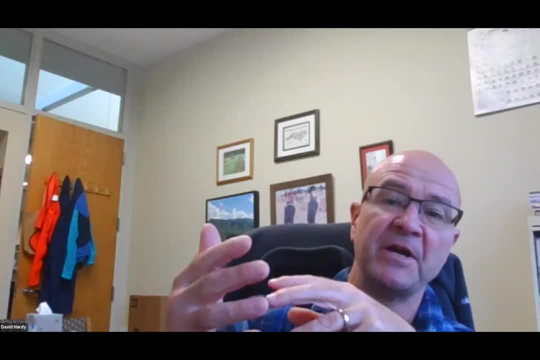 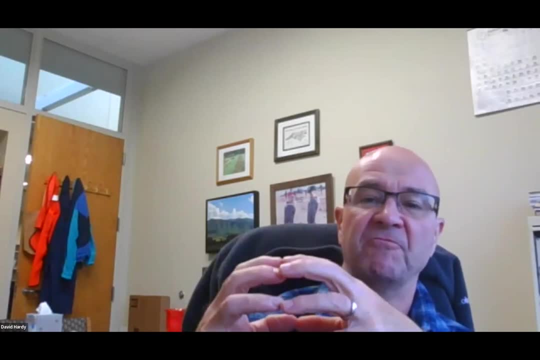 We also have a lot of chloride from potassium chloride being applied Also, nitrate would be leaching. So it's just to comment: not only bicarbonate would be a facilitating anion, but also chloride nitrate and so forth. from that standpoint too, 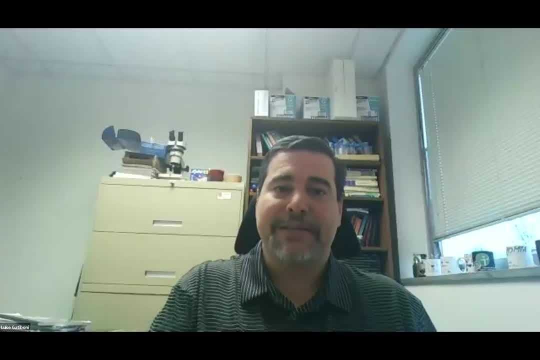 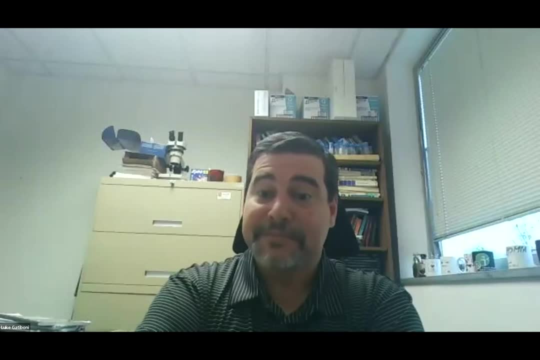 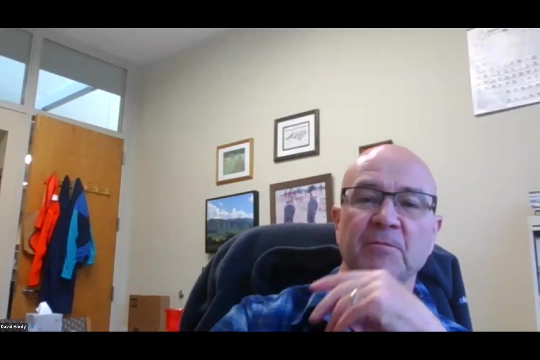 Yeah, this is exactly true. Yeah, the bicarbonate is that one that is linked to the other causes, but all the anions will do the same, And you focused on bicarbonate, which I hadn't really thought much about. I was thinking more chloride and nitrate and so forth. but excellent, Yeah, thank you. 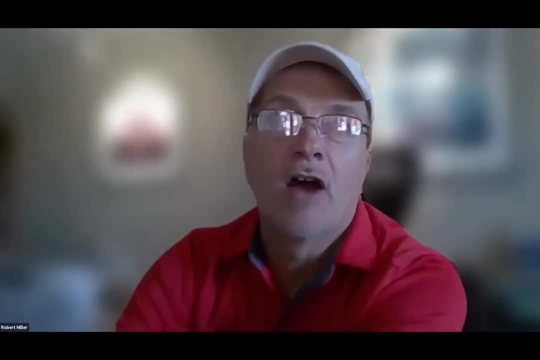 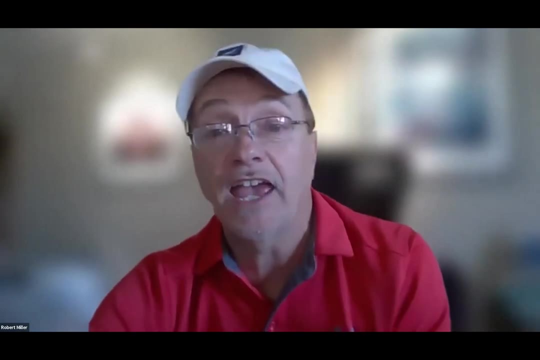 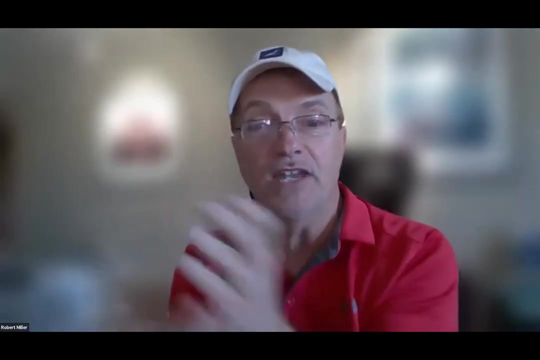 So I'll spin this the other way. So now we start talking about the removal of cations through leaching, but now we also have the cations removal when we cut off corn silage and alfalfa hay, right. So now you're taking all that calcium magnesium and granted some potassium off the field every time you take that, So those cations are no longer in the system to buffer it. 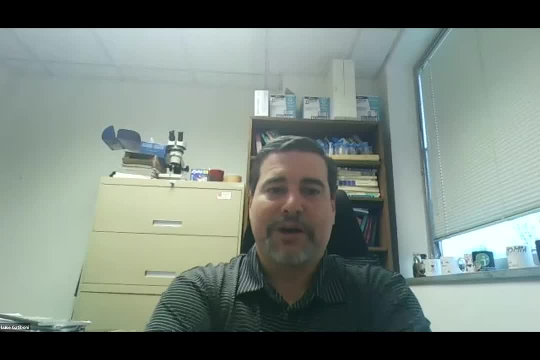 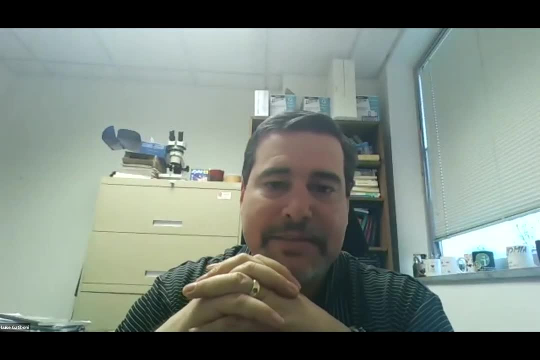 Exactly, Yeah, Yeah, This is the other side And we also have the same process because we have this unbalance of the cations and anions in the system. I think one more thing you mentioned too, Luke. that kind of hit home with me. I think our lime rates fall short from Some of our heavier, more fine texture soils And you know, once we get into the 5.4 to 5.5 range and on up, you showed a very nice linear relationship with increasing, with adding lime and so forth and increasing pH. But I think we have some work here that needs to be focused on especially our heavier soils, many more fine textured and claved soils in that 4.8 to 5 range to get enough lime to get them up to the target pH. 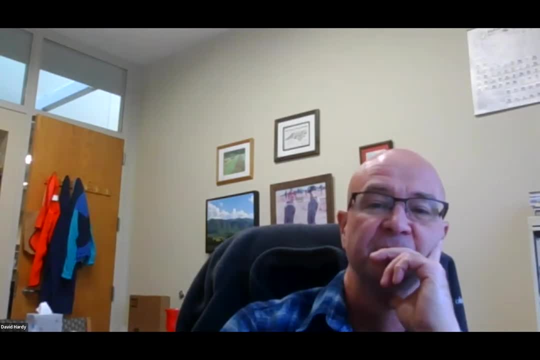 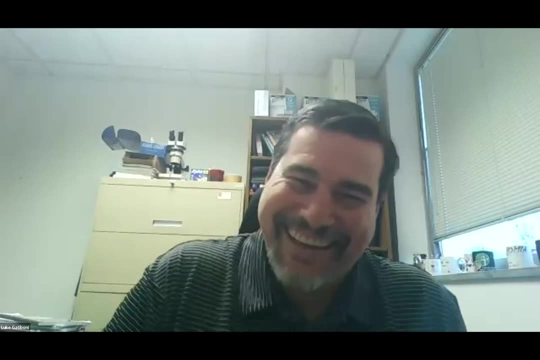 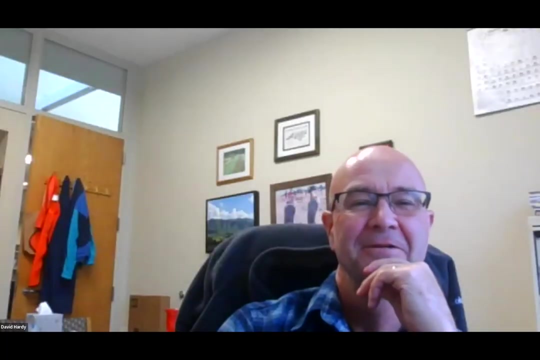 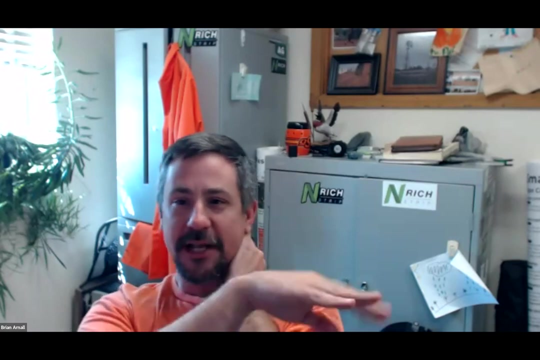 So that's something I think That we are seeing here, based upon some studies we've got. So that'll be some future work for you, probably. Okay, I will put it on my list. All right, Dave, I'm glad you're seeing that, because seeing the same thing in Oklahoma is that once we get that pH, we have a completely change in the curve. 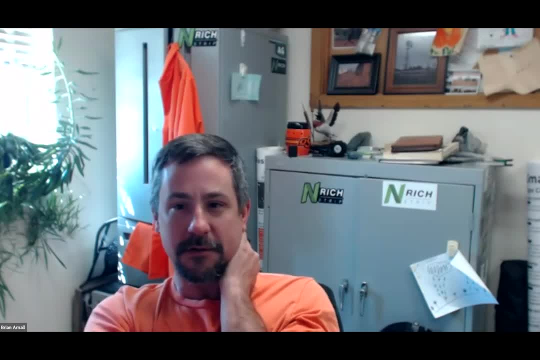 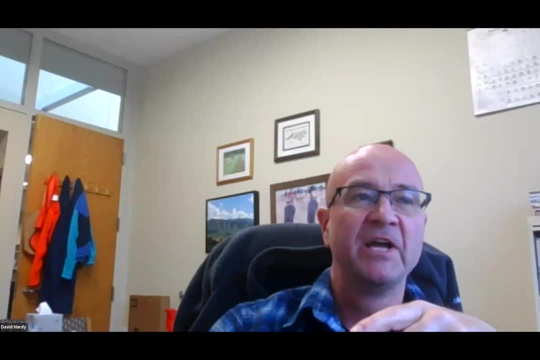 It's like we should have a linear response to a point and then another linear response, and we're not doing that. We just have a single response And for us- I think you know, part of it is not really having the effects of aluminum toxicity, maybe at a 5.5 or above. 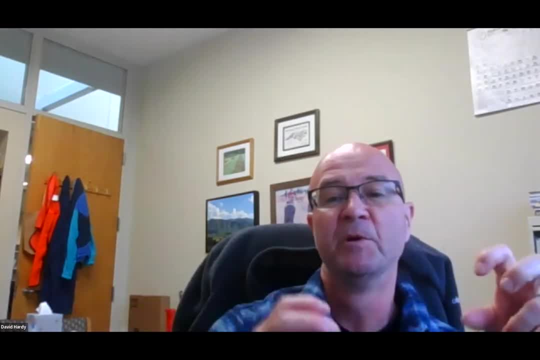 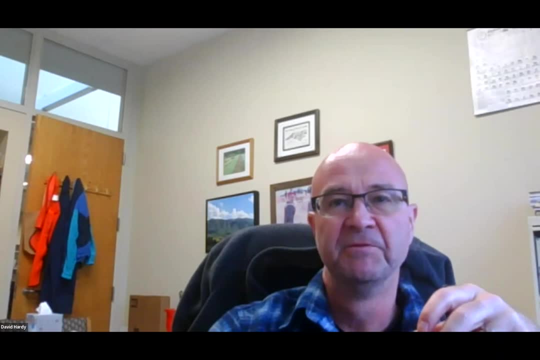 You're satisfying the pH and not having aluminum toxicity. And we have a lot of growers that sample every year. So they sample this year, they get a lime recommendation, They sample next year and may still get another lime recommendation because they are sampling every year. 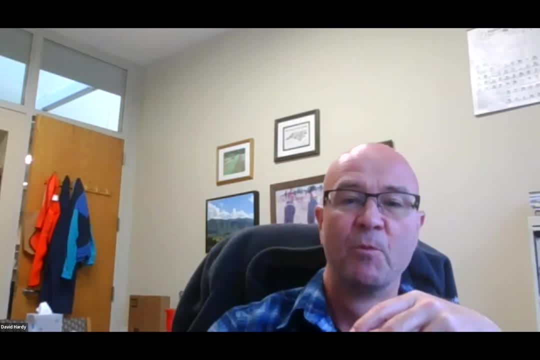 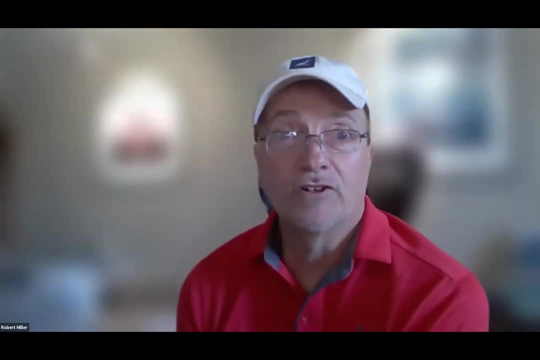 And probably we stay ahead of the curve with that aspect of it, But we're still. We're still not really getting to the target pH we desire. Yeah, And two: most all our buffers- I'm sure even the Malik- were all designed around the fact that working between that 5.5 and 7 range right. 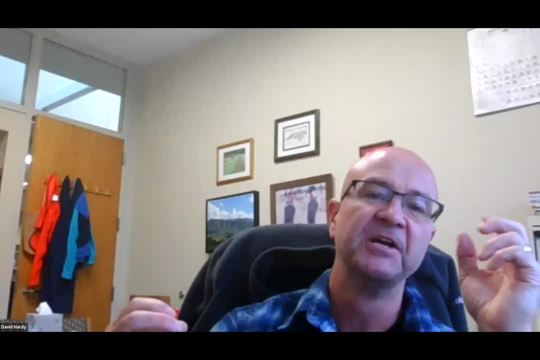 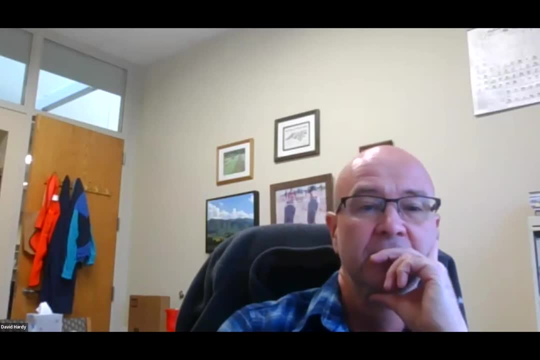 Yeah, And Camper that really looked at a target pH. he was looking at trying to minimize the effects of aluminum toxicity is what his work was geared toward. Yeah, I can give you an example from our subtropical soils in Brazil that we have a lot of. 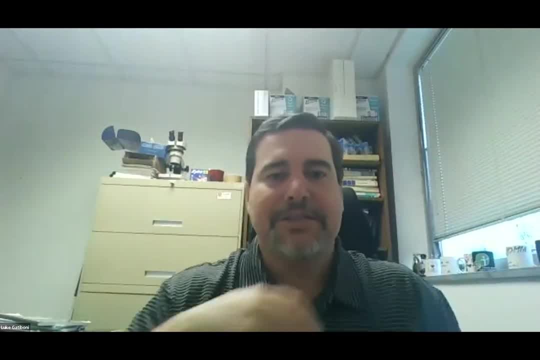 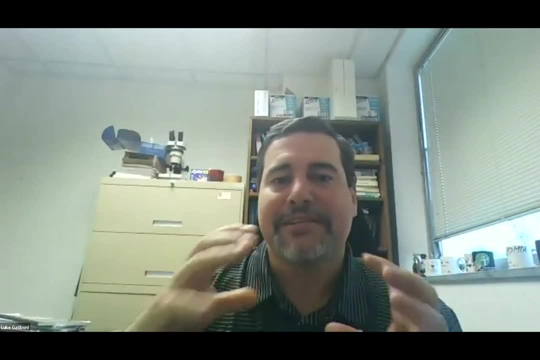 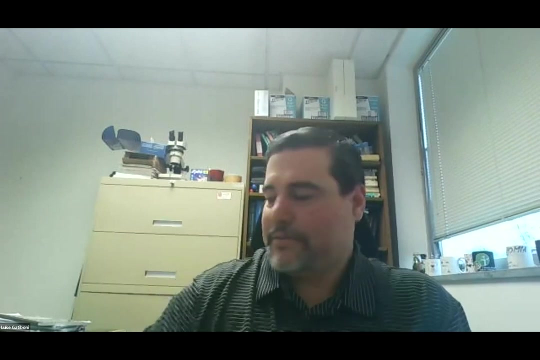 We have a lot of aluminum and we start with a very low pH in agriculture and we can already use a linear equation. We use other types of equations because we have this high buffering capacity at low pHs. Any more questions? Yes, Go ahead, Frank. 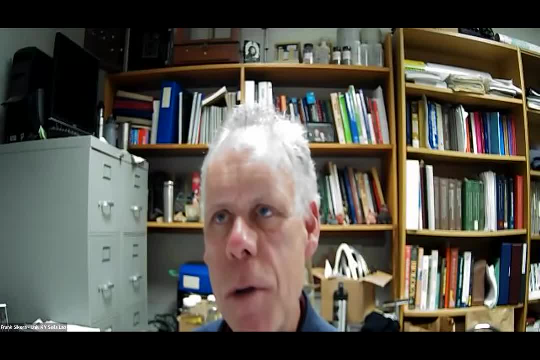 Sorry, I had a comment, just something that kind of bugged me on the terminology that we use in soil chemistry, And when I taught plant-soil relationships I tried to teach the students that cations aren't really bases. You know, if you look at it from a chemical point of view, a base is something that consumes a proton or consumes acidity. 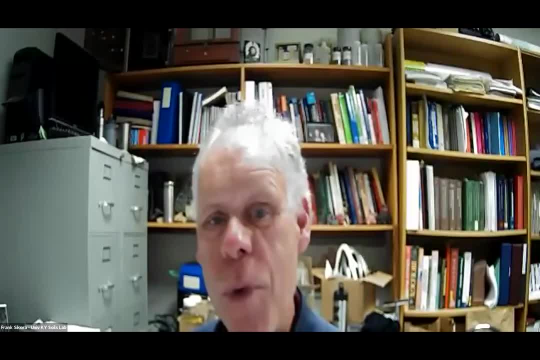 Yeah, yeah, yeah, You know we call these base cations, but they're called base cations because they're not acidic. You know it's a hard thought to have to try to get across from a chemistry point of view. 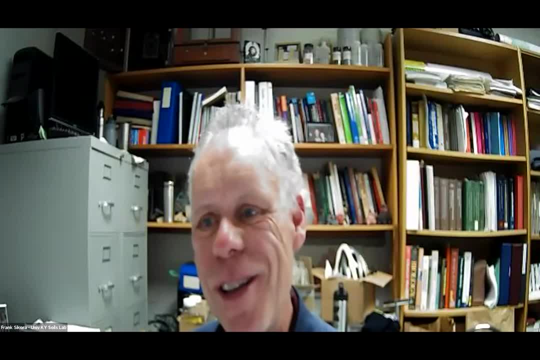 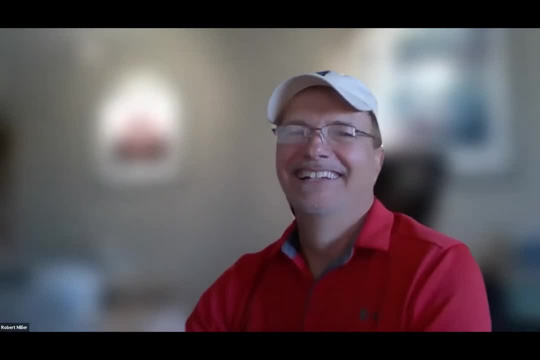 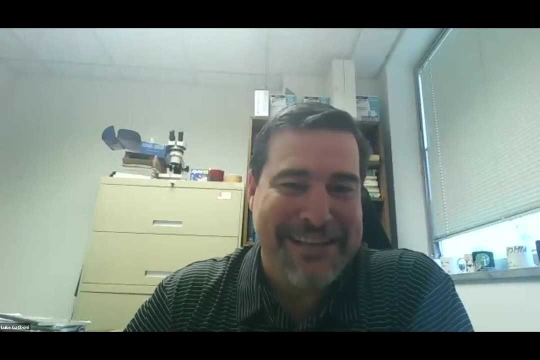 But you know just how do you approach that Lu. Do you touch that at all? I try to avoid. but I know that I try to avoid using basic cations, but sometimes I just forget to use this terminology. But I agree with you. 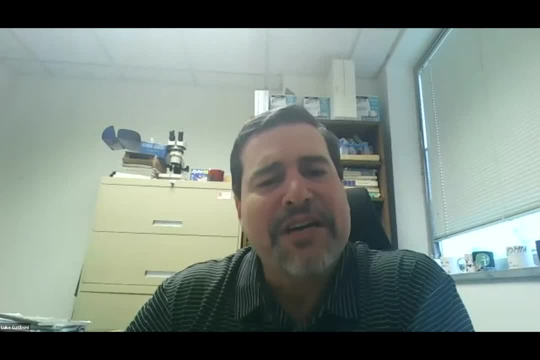 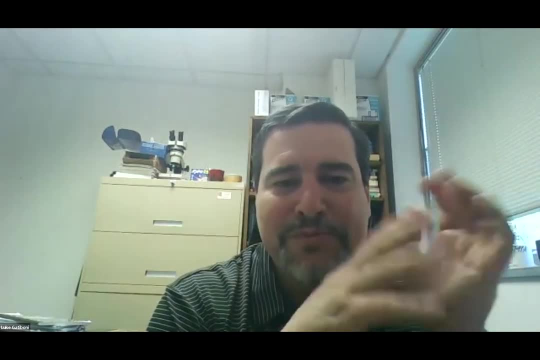 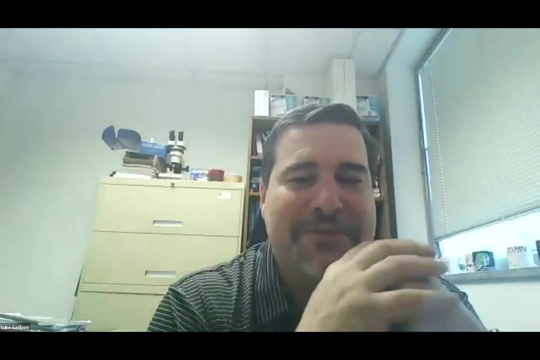 It's something that causes a lot of confusion, And I think the origin of this is because we have the periodic table. The first two groups are basic alkaline ions elements, And so this basic I think comes from there. But it's just confusion. 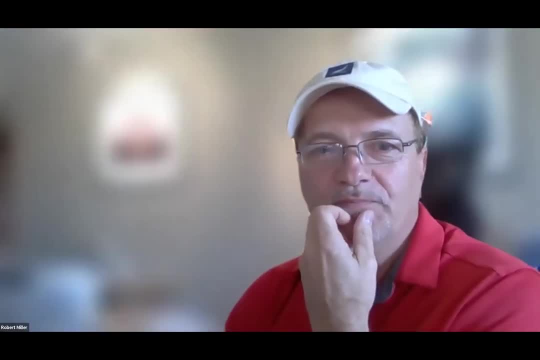 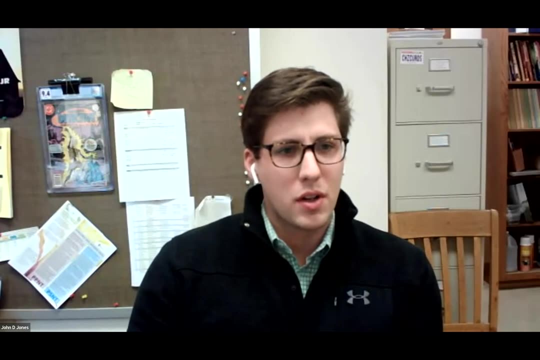 Thanks, Okay, any more questions. I think John did. I just wanted to group And we just started a study here on kind of a liming rate and frequency of application And we're trying to get across that correcting the pH up front with one application might have more value than trying to do small annual applications. 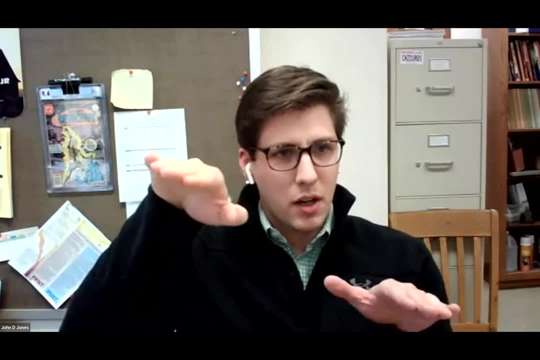 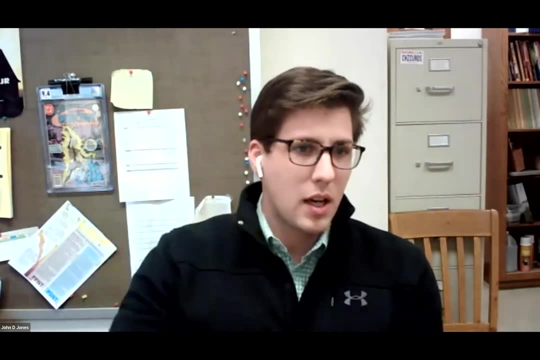 And that the point of the curve before it turned linear kind of got me to thinking about that, because there was more acidity to neutralize than at a higher pH. And so we're, you know, starting in In pHs of 53,, 55,, essentially. 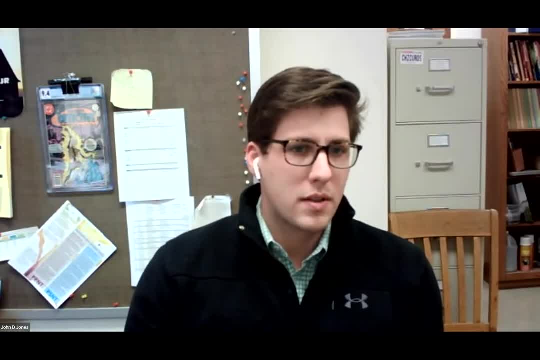 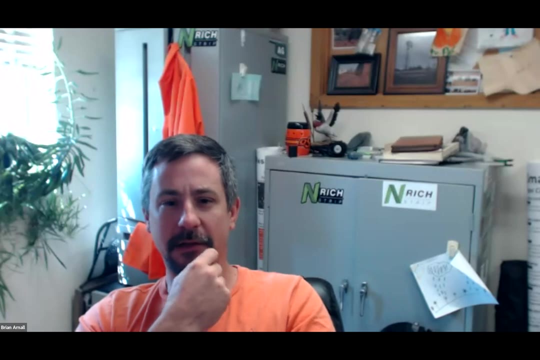 I don't know that might might lend to considering that, but I'm skeptical of low 200 pound CC applications every year as being effective as correcting it right away. going forward, John, what's the rationale of low right, multiple year that's? that's something we wouldn't ever recommend in the southern whites. 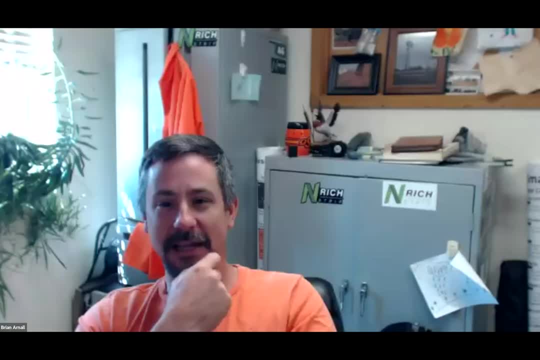 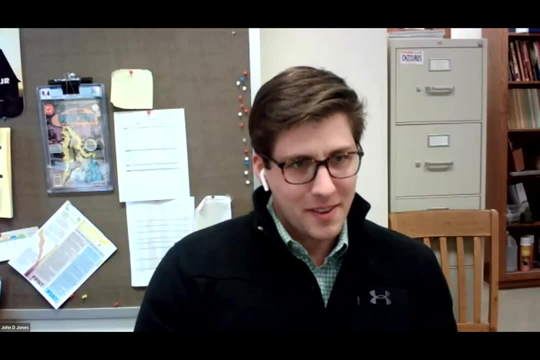 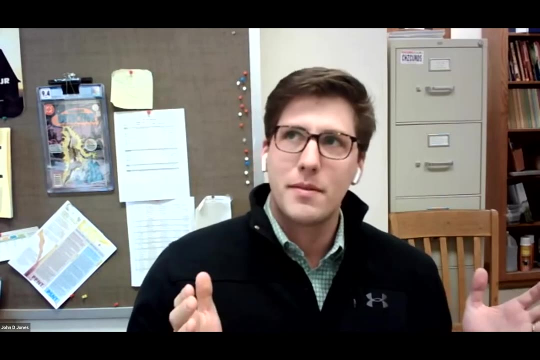 So I think it's coming down 1000 pounds. We say: don't run it. I think it's coming from a pellet and lime sellers. That's fine, Yep, And so that's that's what we're, you know, comparing some source product to, but I think that's you know. you know trying to sell, banding it in the row or something like that. 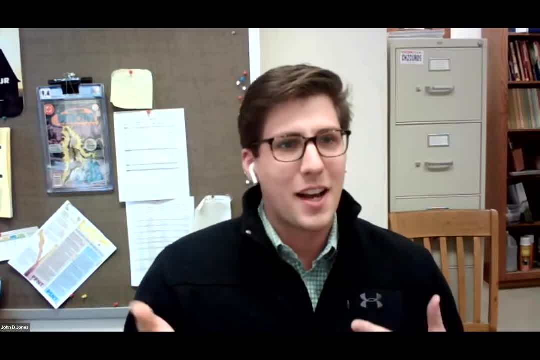 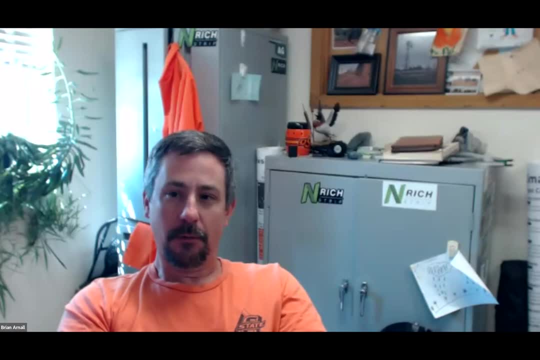 It just- And unfortunately I saying it, not having the data isn't as powerful as us having a small two year experiment to show the data. but, John, I don't know if you've seen it, Sorry, go Brian. So you saw Jeff Edwards and this was Romulo. a lot. 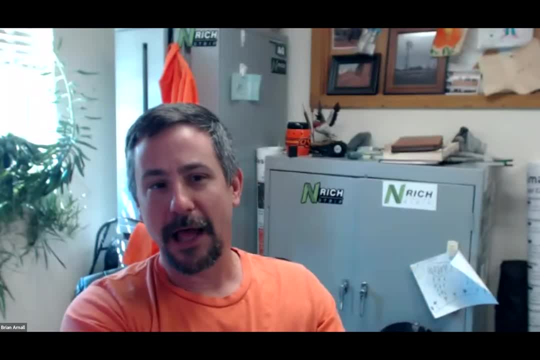 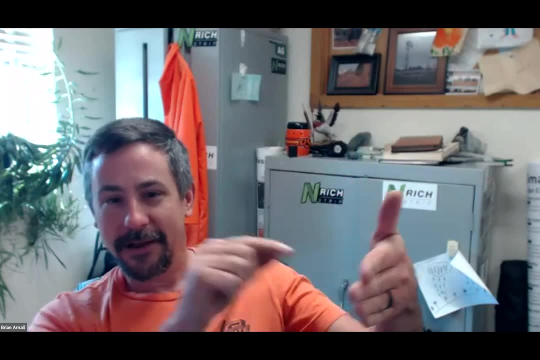 Oh, who's not case state is doctorial program. looked at liming, the banded pelletized lime, and they've got some beautiful post harvest stratified and going in. you can still find that pellet posts tweet harvest. so A picture of state in my mind. 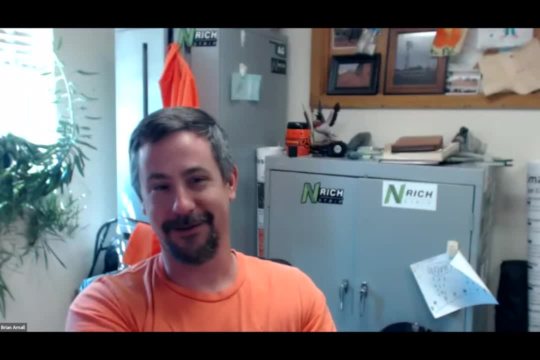 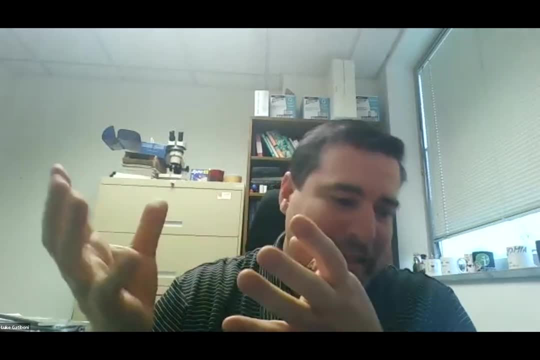 What I would have seen it john said, just saying that I use that all the time And you know. remember that these of the acidity is a dynamic equilibrium. If you don't apply all the lime at the same time, you'll have the soil buffering again. 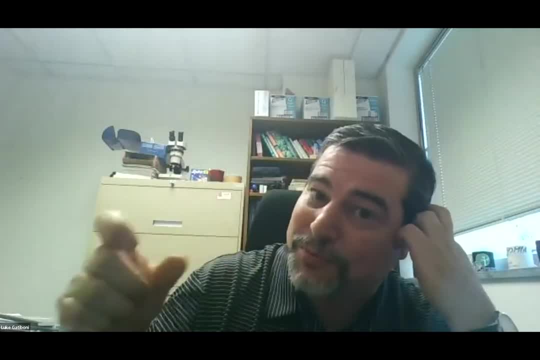 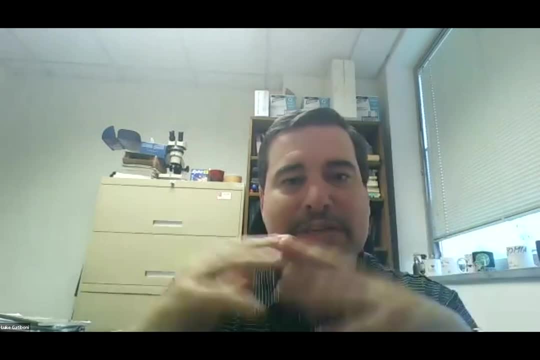 and then you'll drop the pH, And so for me, it doesn't make sense to put these small rates. Maybe the only situation that I would think about this if you are using an O2, that you don't have this lime incorporating the soil. 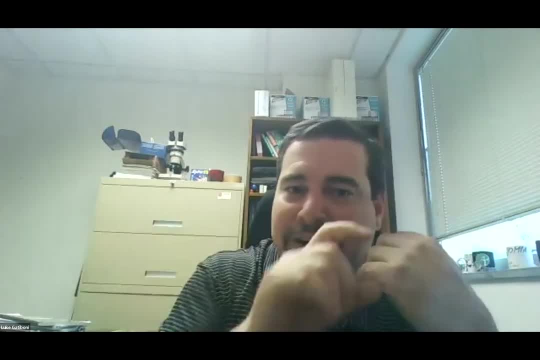 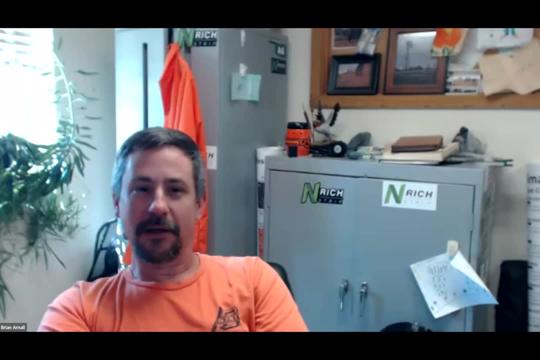 and so a smaller rate makes sense, because we are not neutralizing all the top layer of the soil. I don't know- I want to bring that up because Luke said it. So how many of you guys have a no-till versus conventional till? lime recommendation? Good one, Crickets. Okay, well, that answered my question. Thanks guys. So I'll go spin back to John. My point is about the pelletizing, The pelletized lime. you know, 200 pounds of the acre every year. 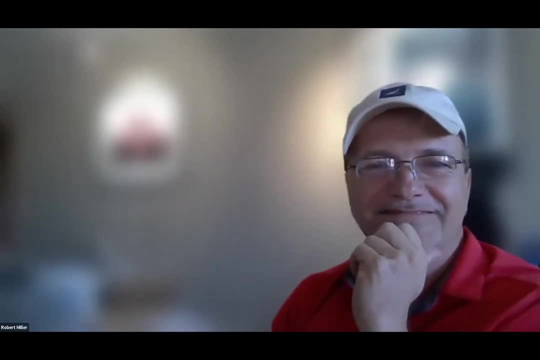 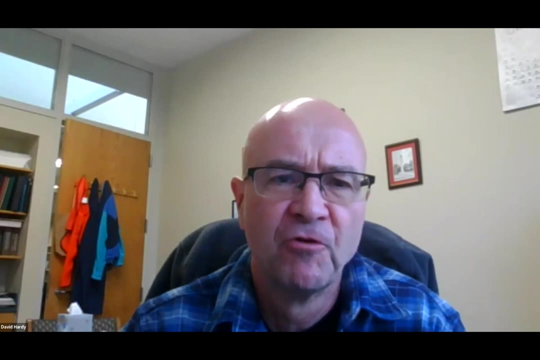 That's guaranteed product sales every year. That's what it's about. One thing I would comment about that too. with pelleted lime you're looking at very small particles. You don't have any reserve larger particles to carry through for maybe two or three years. 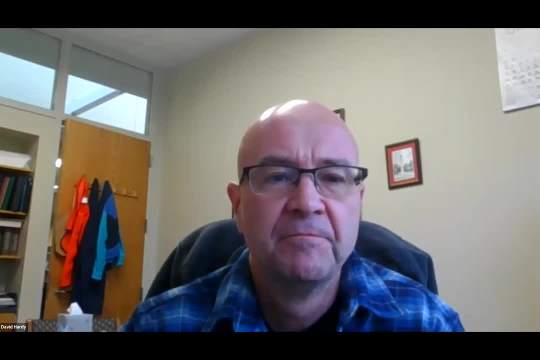 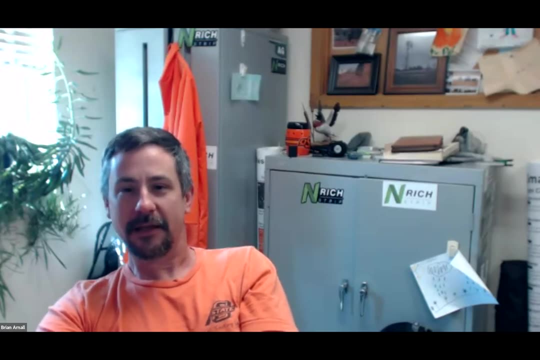 to help you know, continue pH where you want it to be. Bob, we've also seen so the pell lime that every year in the rate is more associated with current prices of grain and other thing. What would be less than an application of lime? They're going at a percent what you would take to apply lime and they're cutting it so that you don't have that same lime cost. And so if one costs you $50 an acre to fix it, they're going to sell you a $15 an acre product every year. 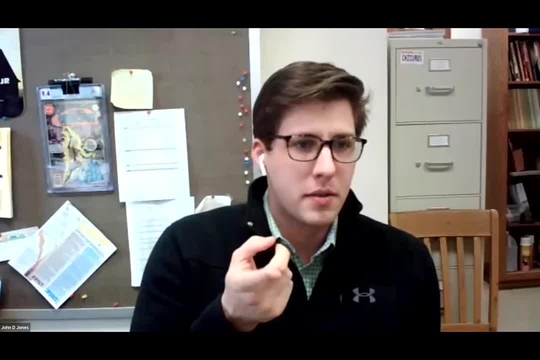 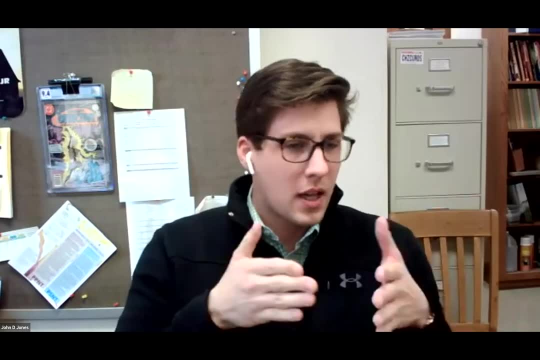 There you go. So that's what I'll bring this up. I'll bring this up next month too, But that's what we found is that on an effective CEC basis it's the same, It's same rate as needed. So it's, you know, it's there. 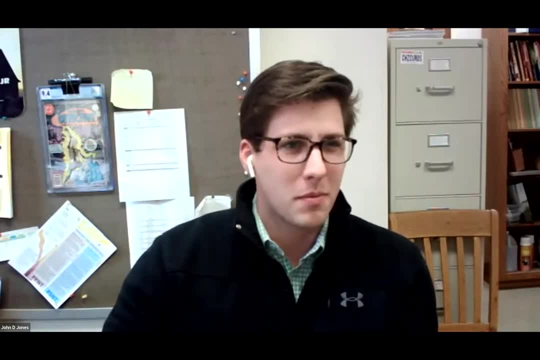 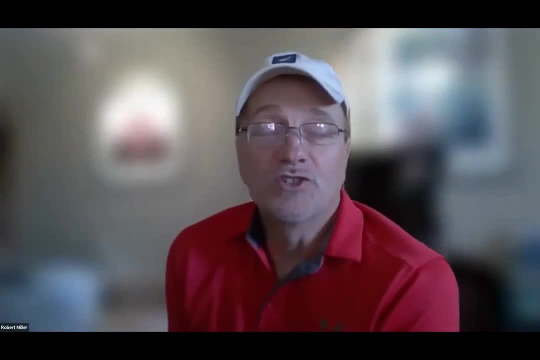 They're trying to sell the product, not the analysis, maybe, or something like that. There you go. That's what it's all about a lot of times selling the product, Guys. I've really enjoyed this discussion and everything, And I think we did a nice, nice leap into the next session. 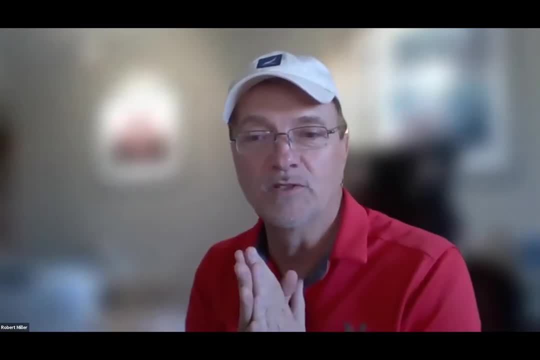 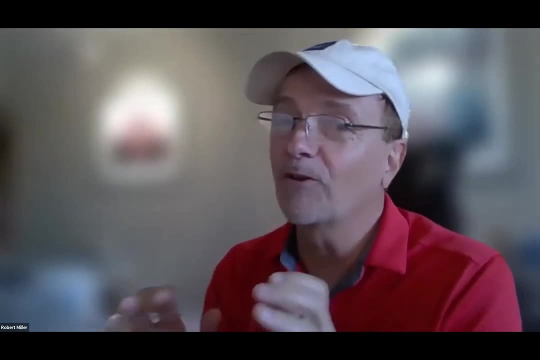 on May 16th, talking about what John's going to talk about in terms of incubation studies and liming. I mean, I'm sure, knowing the group that we have here, we could go on for quite a while about this, but I want to kind of wrap stuff up here because it's coming up in the 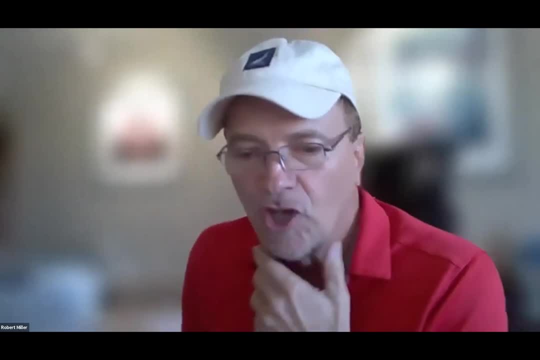 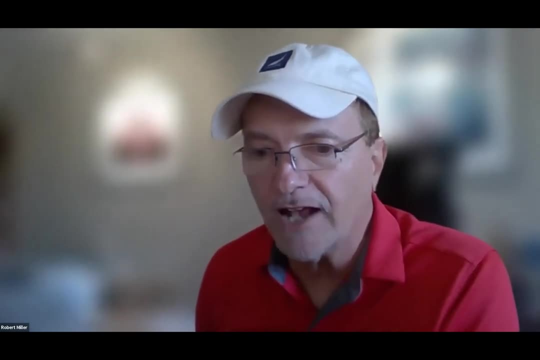 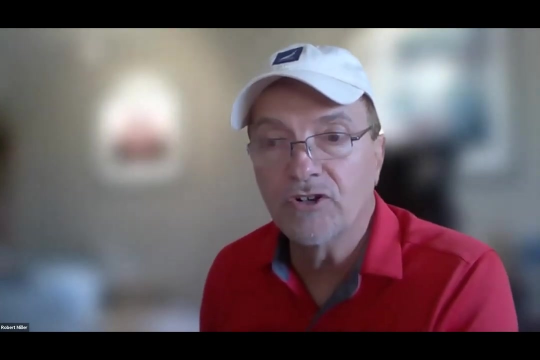 top of the hour. So so far I have 17 lab- or sorry, 17- results from different land grant universities on the lime racks. I've got about another eight or nine that I'm still waiting on and I'll have that wrapped up and I'll circulate that out to the group soon as I. 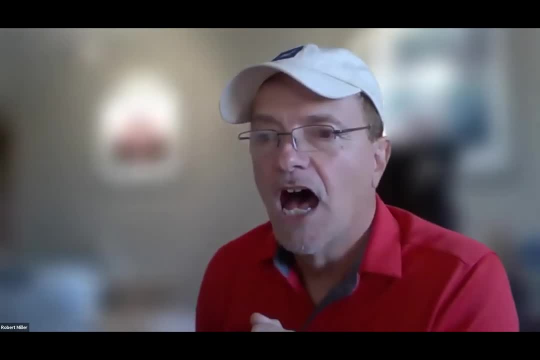 get that. The last one's pulled in on that. One other thing that's in the mill: For each one of our presentations I want each one of the authors to come up with four, three or four papers that they think that really talks about what their 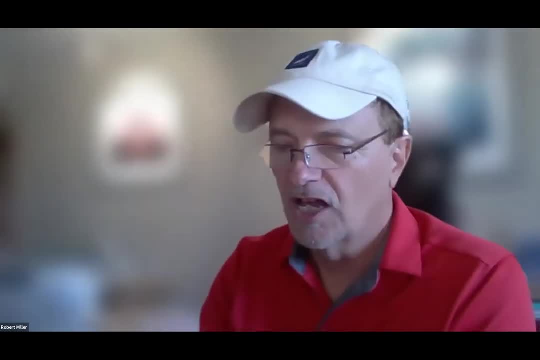 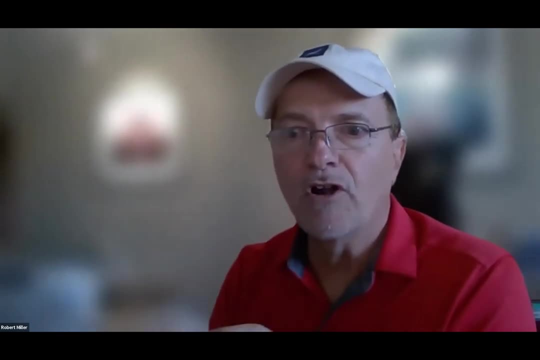 focus is in terms of pH for David Buffers, for what Frank Sikora talked about, what Luke talked about today. I'd like to kind of build a kind of like a miniature library, that for people who don't make our sessions and we get into a topic. 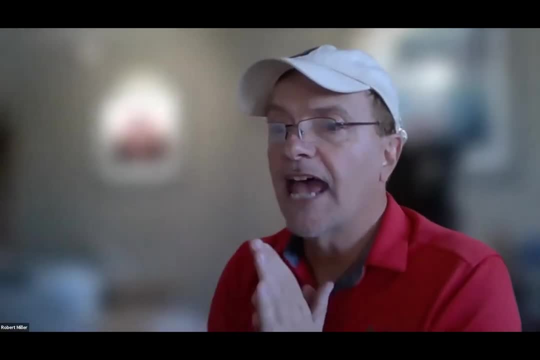 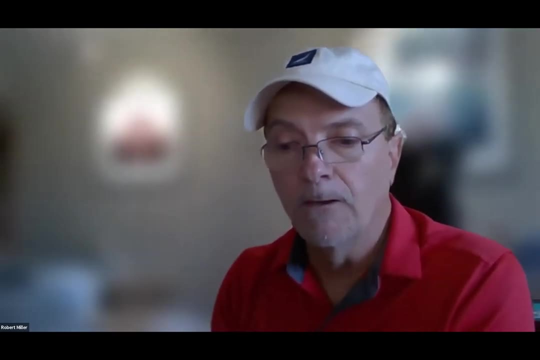 we can have that as a reference. The last thing we're going to start working on the next step. The next step, once we get done with our presentations next month, is to jump in and start developing a project, And I've got a little group right now that I'm putting together to talk.